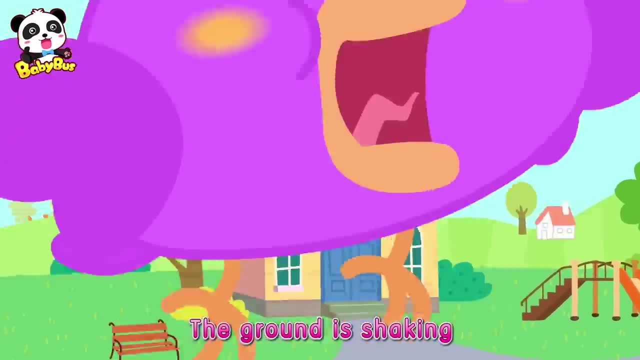 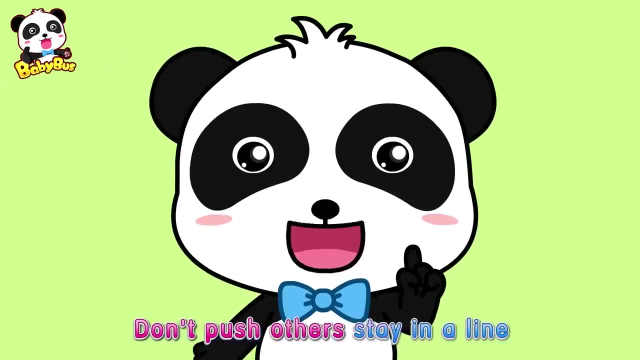 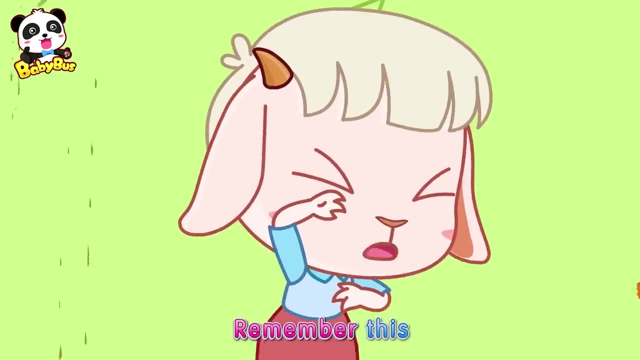 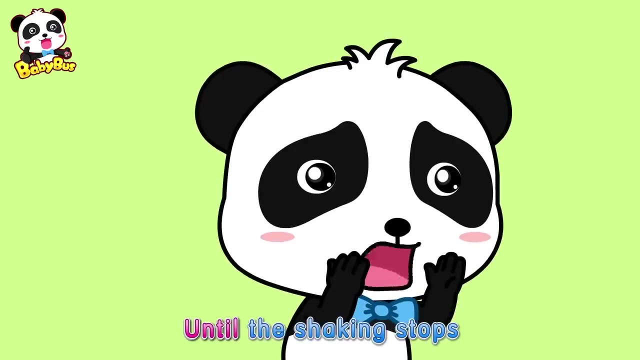 The ground is shaking. The ground is shaking, It's an earthquake. Please stay calm. Teacher says, don't push others, Stay in a line All together. let's go now. Remember this: during an earthquake, Stay in a safe place, Keep calm until the shaking stops. 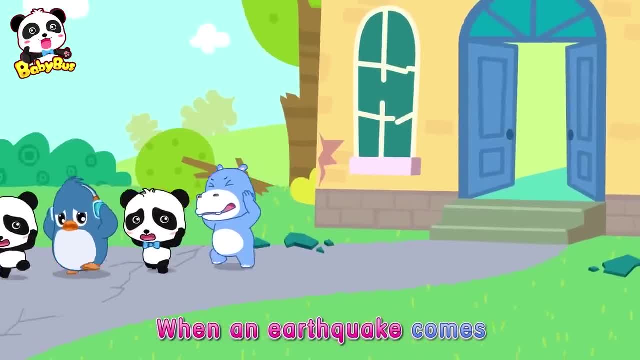 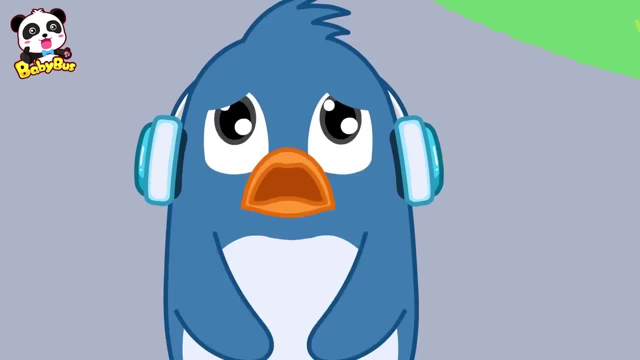 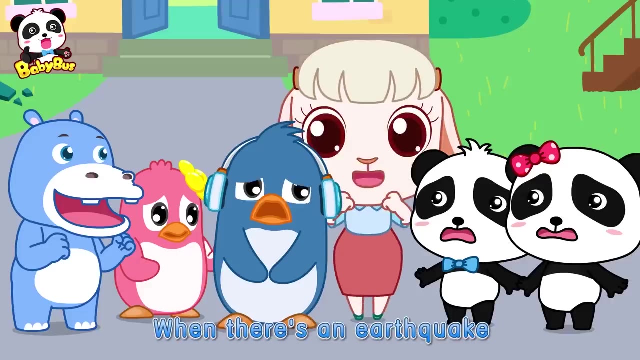 Until the shaking stops. When an earthquake comes, I can protake myself. We're safe now. We're safe now. The earthquake is so scary. I'm so happy that all of you are safe When there's an earthquake, stay calm. 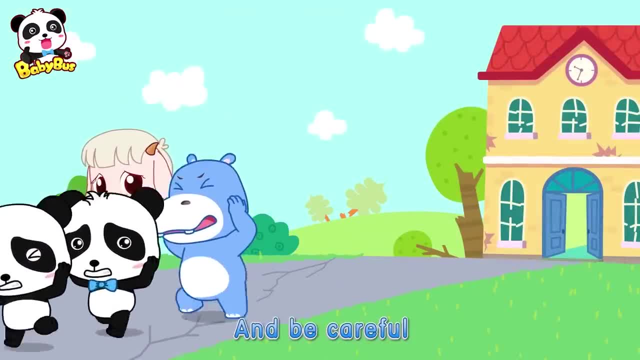 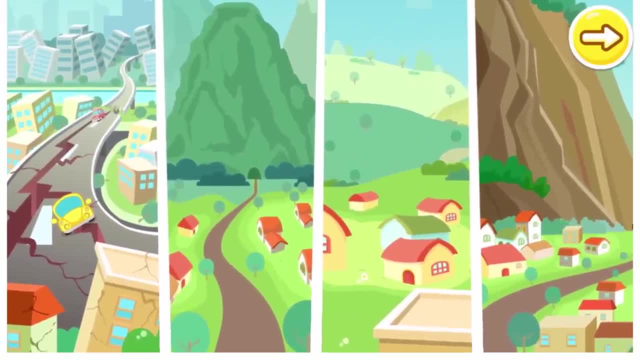 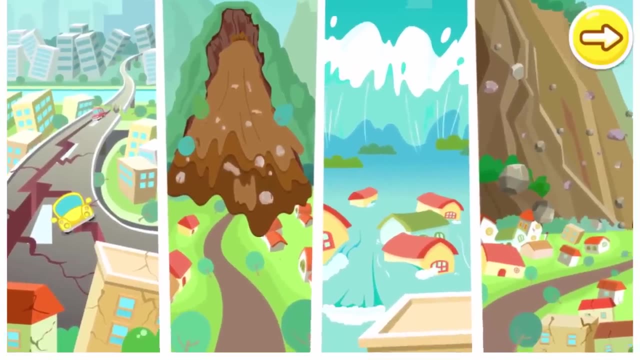 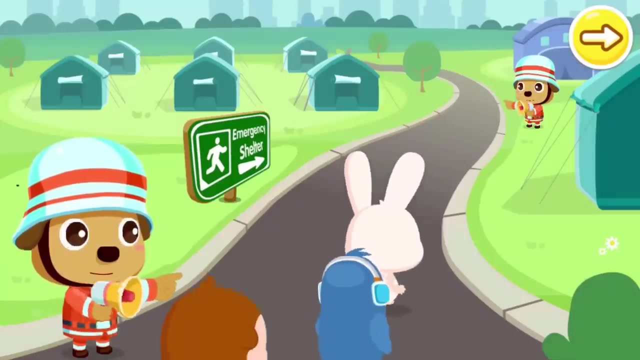 Listen to the teacher's directions and be careful. Please keep it in mind everyone. Earthquake, Debris flow, Flood, Landslide: What if our village was destroyed? after these natural disasters took place, We have to escape to an emergency shelter, following our teacher's or parents' instructions. 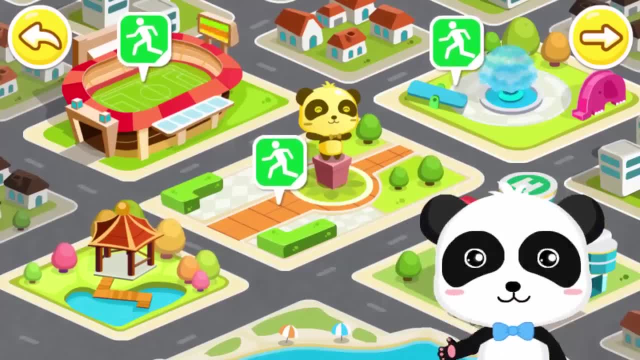 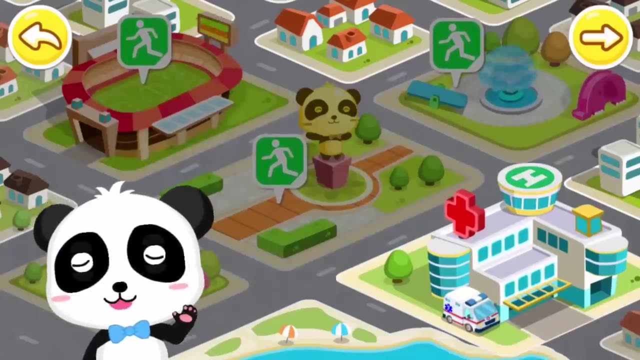 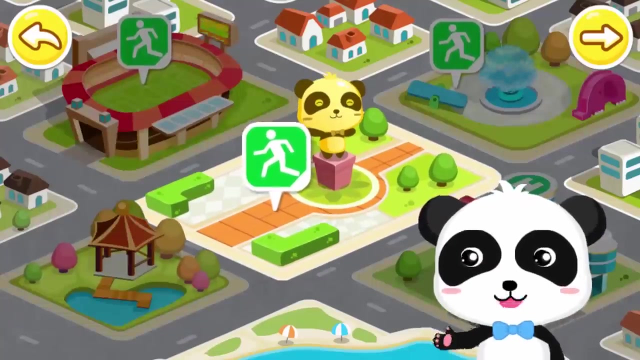 If you don't have a place to go in the event of a natural disaster, you can go to a shelter. But what are the shelters? The hospital is not an emergency shelter. The hospital is not an emergency shelter. Yes, this square has emergency shelter signs. 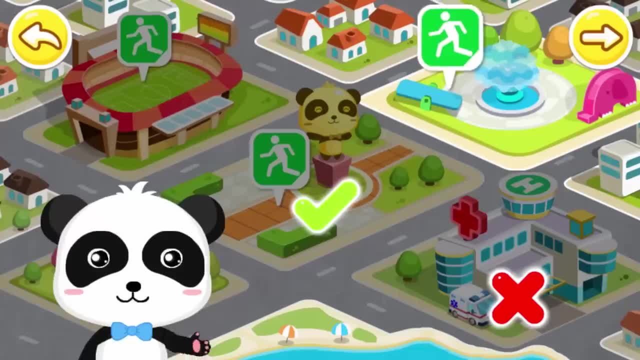 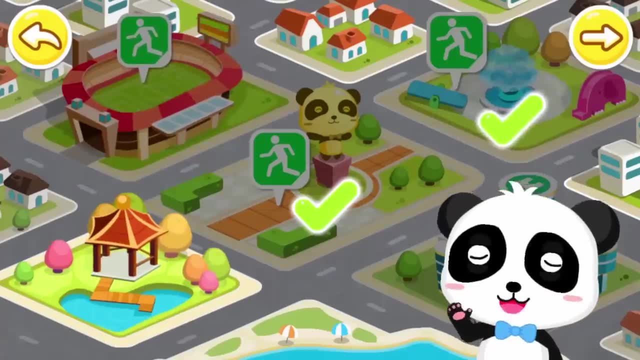 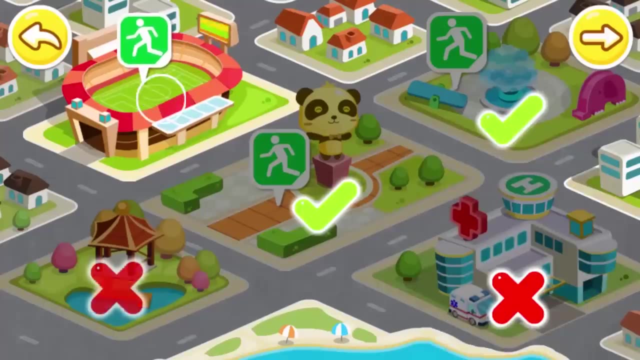 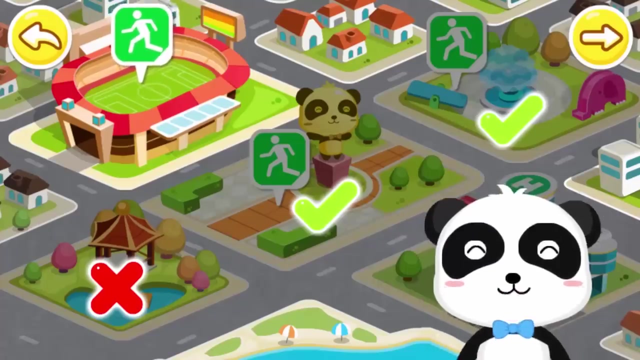 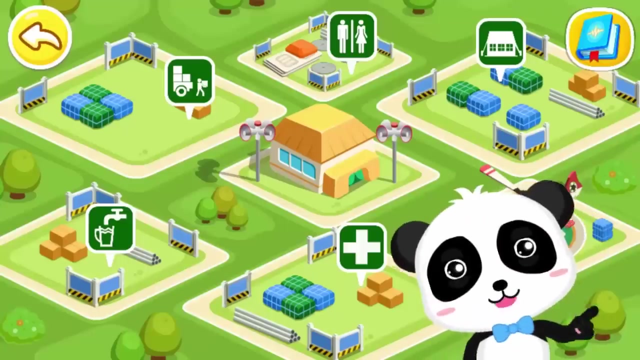 Wow, this park has emergency shelter signs. Very nice. No, this park doesn't have emergency shelter signs. The stadium has emergency shelter signs. Great. Wow, you have found them all. Let's build an emergency shelter. Let's build an emergency shelter. 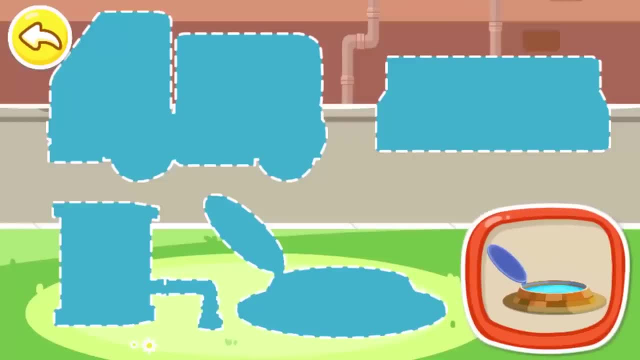 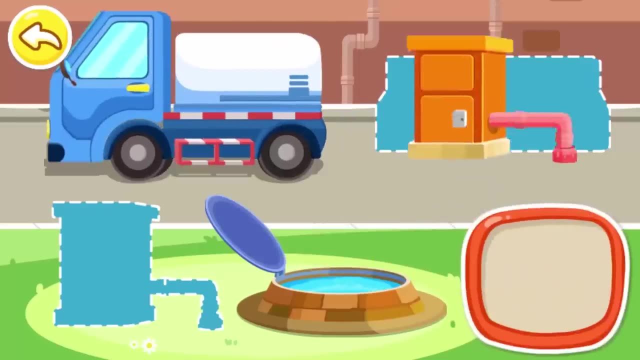 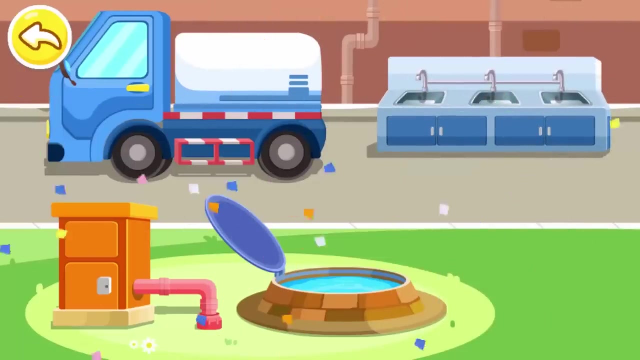 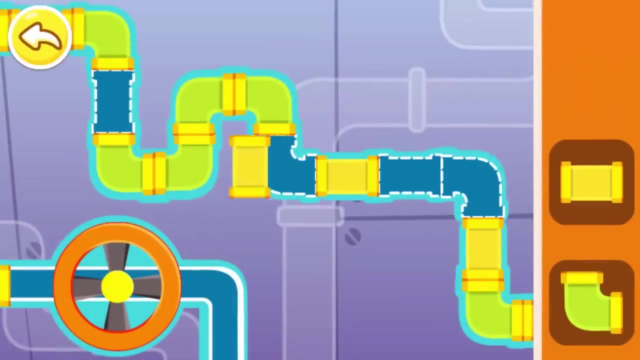 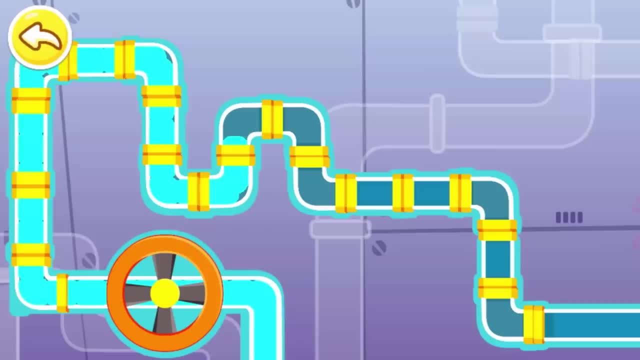 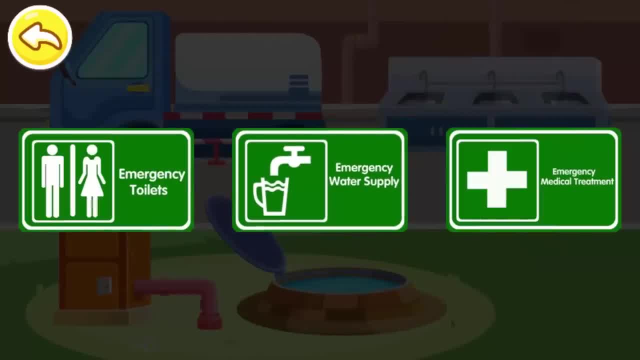 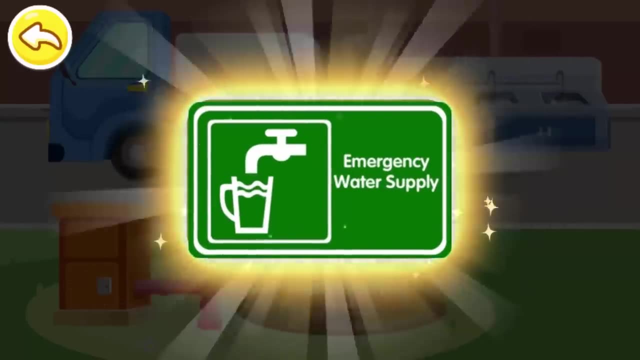 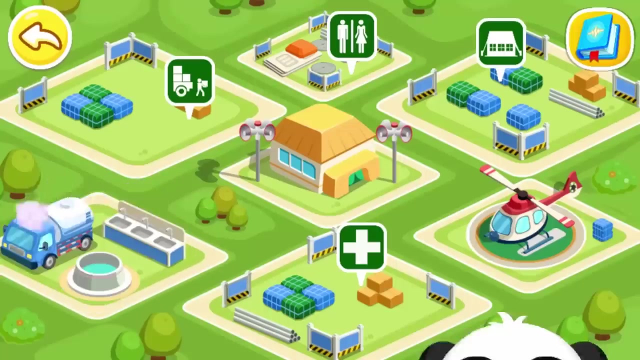 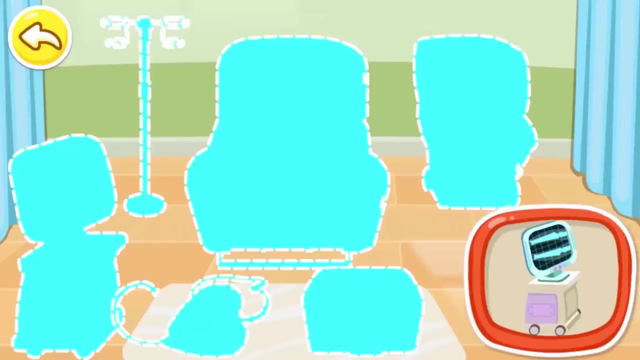 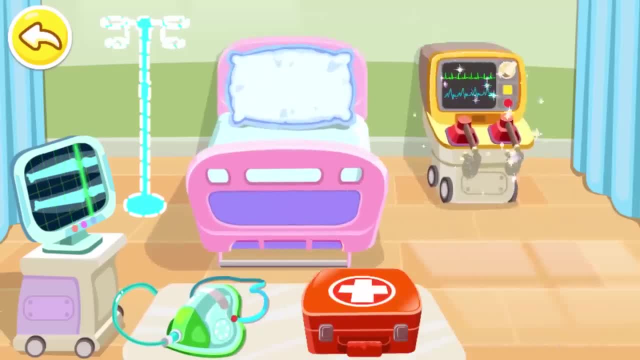 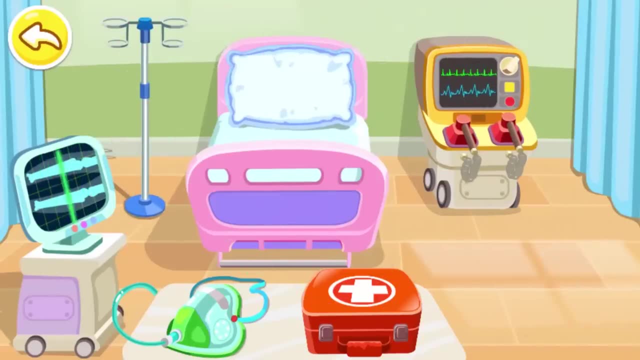 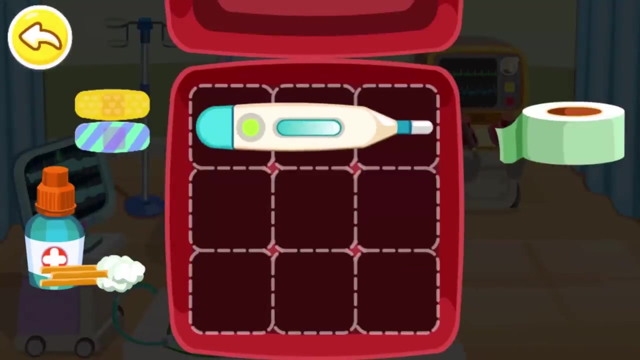 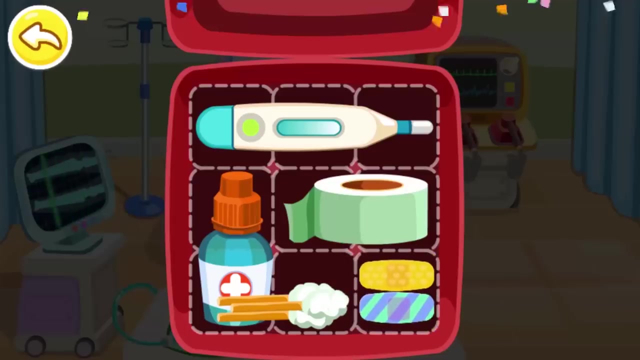 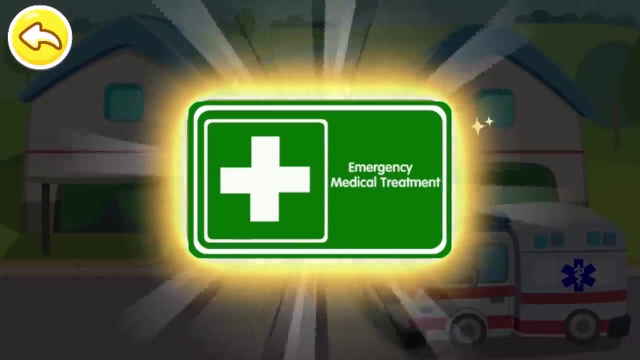 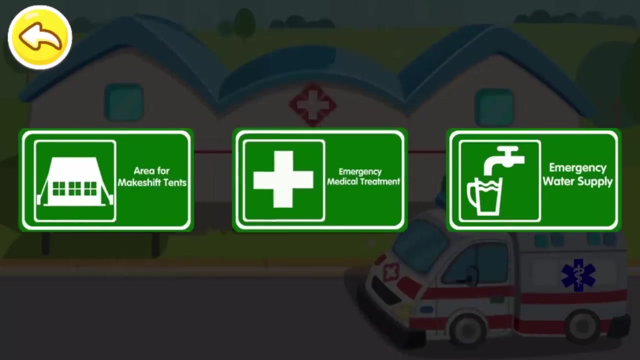 mask bed defibrillator IV pole. let's make up the first-aid kit. here is the emergency medical center where you can come if you are sick or hurt. what is the sign for emergency medical treatment? no, you will see a cross on the sign for emergency medical. 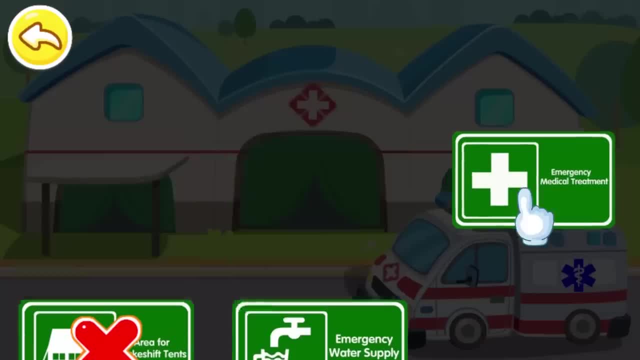 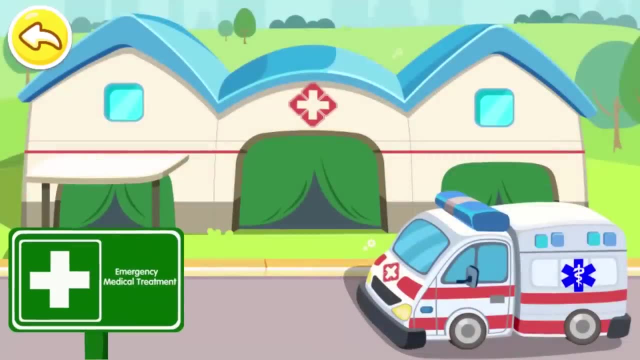 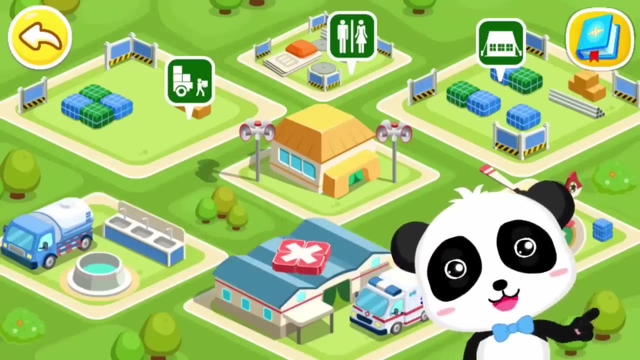 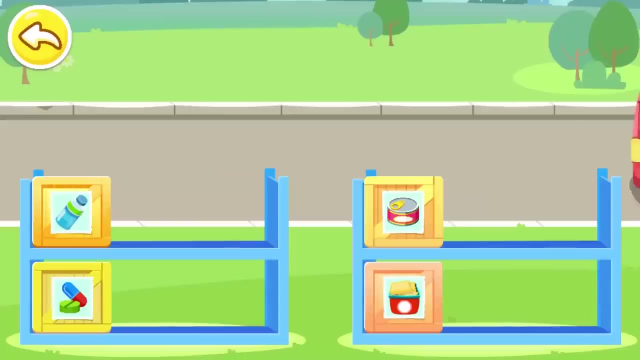 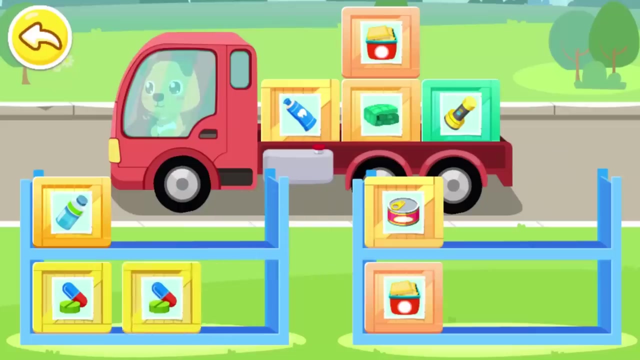 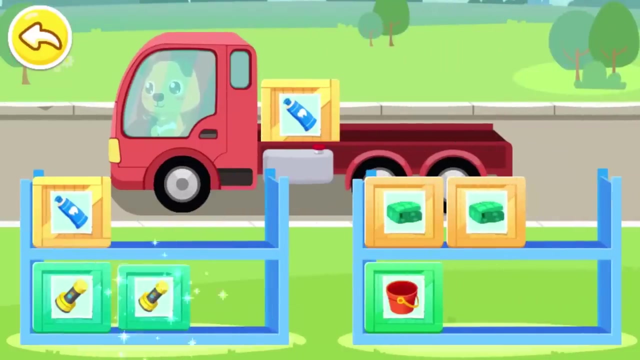 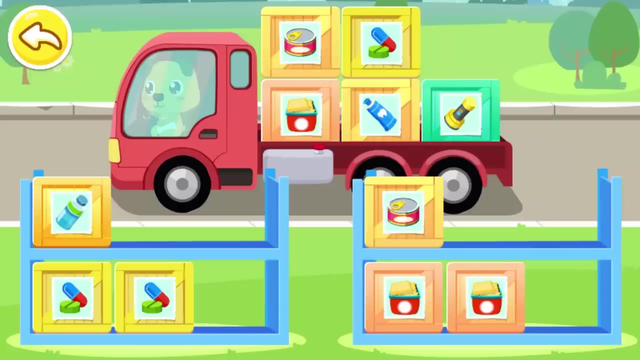 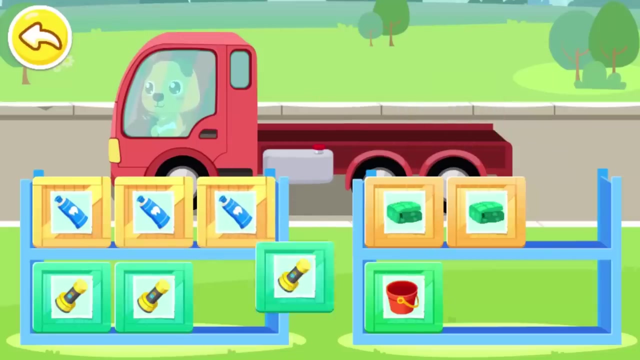 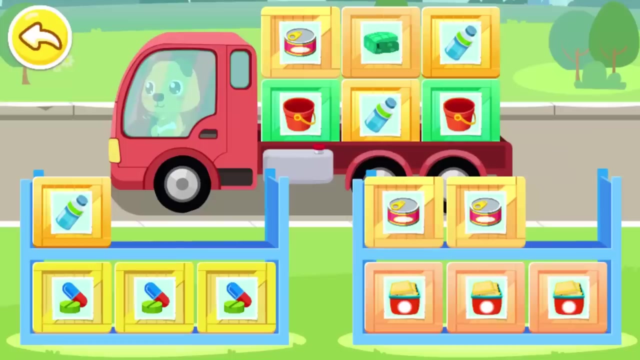 treatment. yes, that's the sign for emergency medical treatment. an emergency medical center has been built. emergency supplies: where should I put these medicine cookies? no, that's not the right place. cookies. well, flashlight toothpaste. where should I put these canned food medicine cookies, toothpaste- flashlight. where should I put these canned food? water, water. 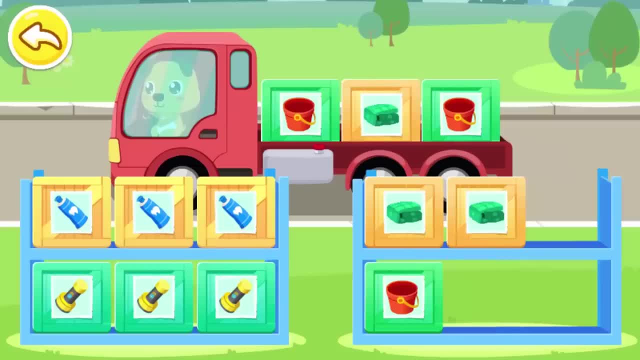 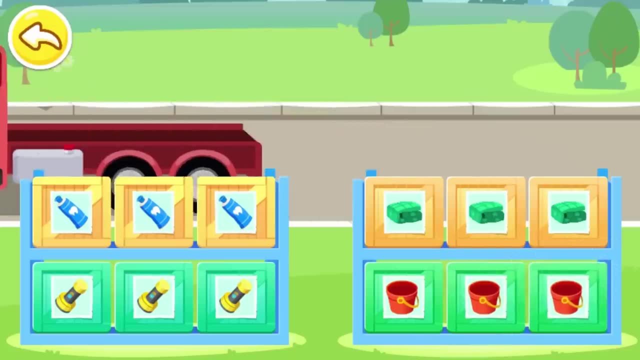 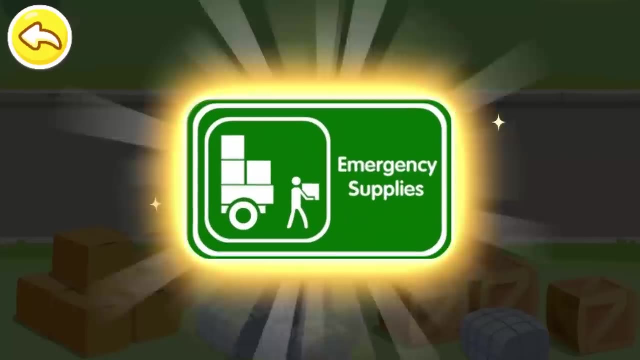 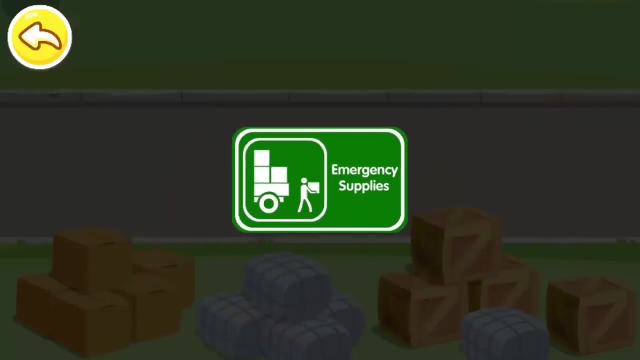 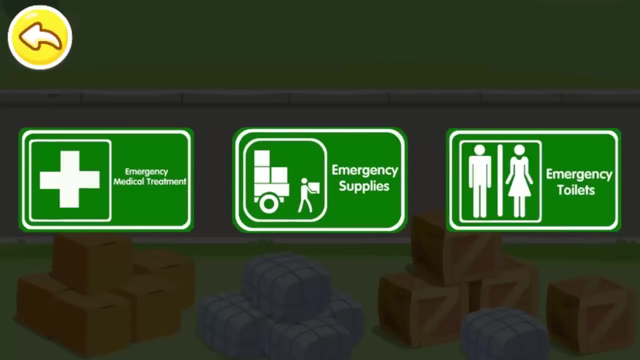 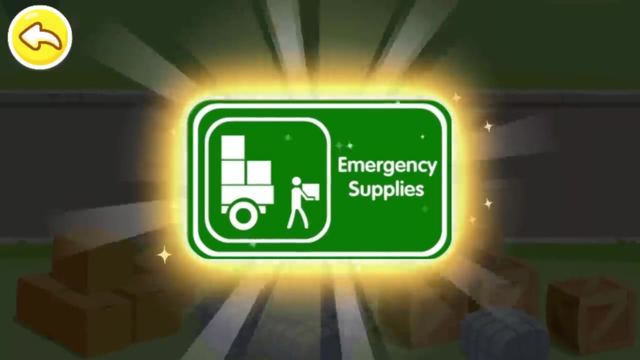 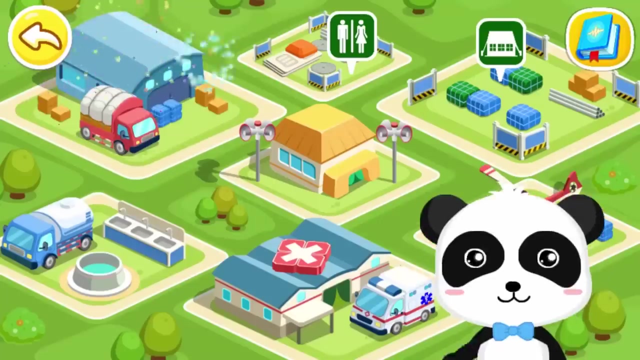 toothpaste, toothpaste. there is a small bottle bottle. here is an emergency supply center. you can come here if you need something to eat. yeah, yeah, yeah. What is the sign for emergency supplies? Yes, that's the sign for emergency supplies. Wow, an emergency supply center has been built. 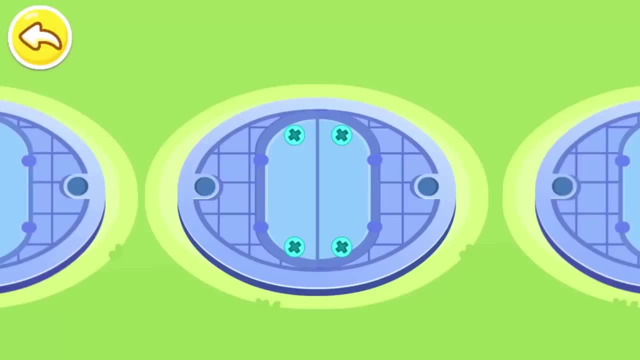 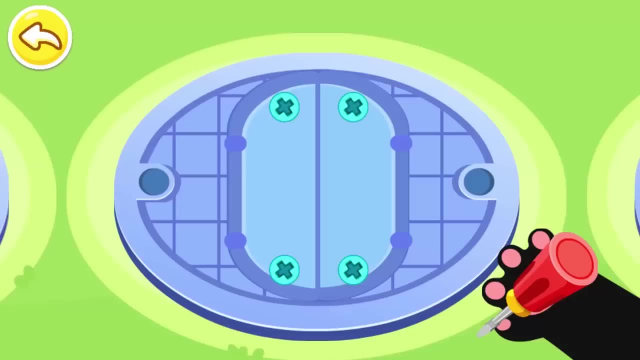 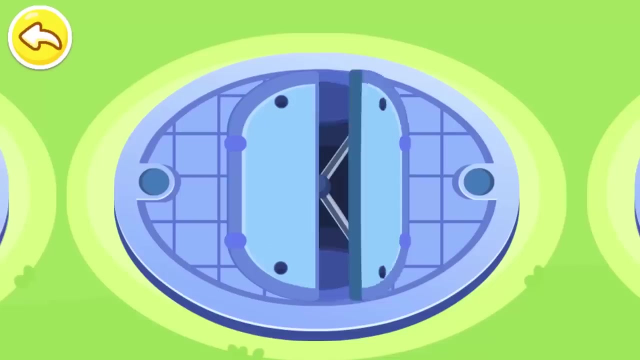 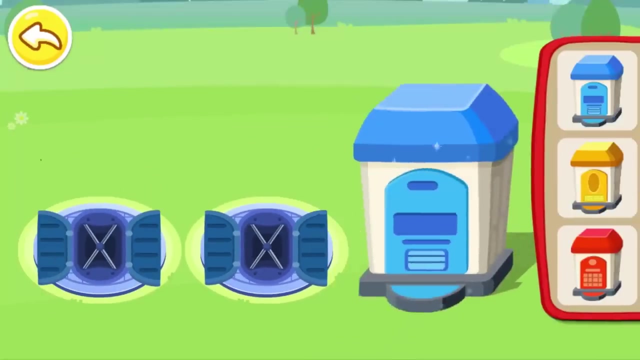 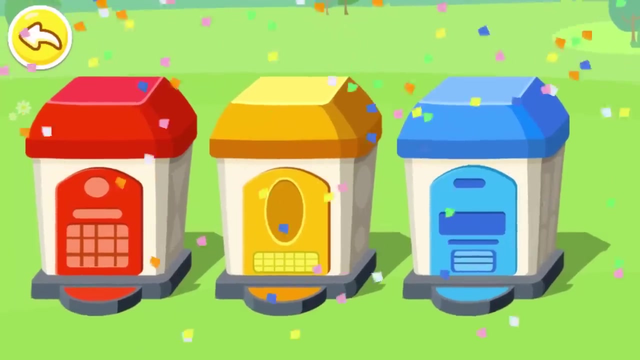 Emergency toilet. The manhole is locked. You should loosen the screws. One, Two, Three, Four. Wow, they are all loosened. Now we can open the manhole. Blue, Blue, Yellow, Red- Wow, you have chosen a pretty one. 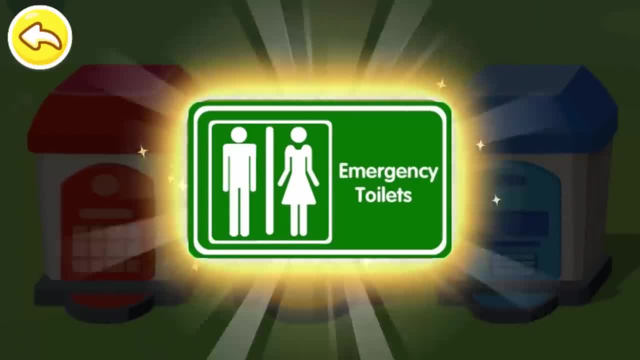 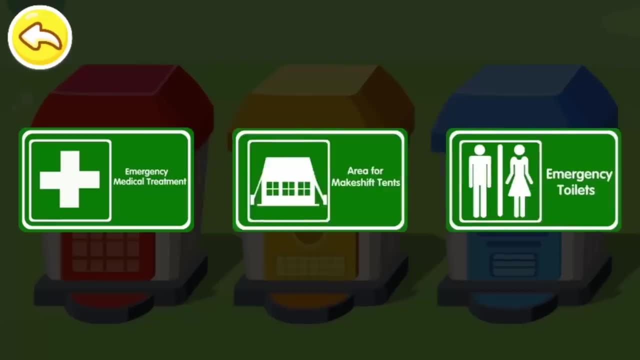 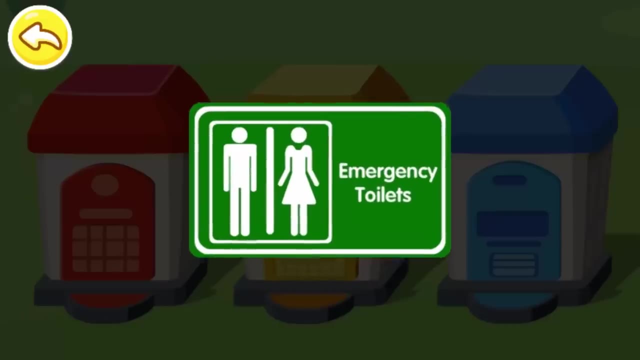 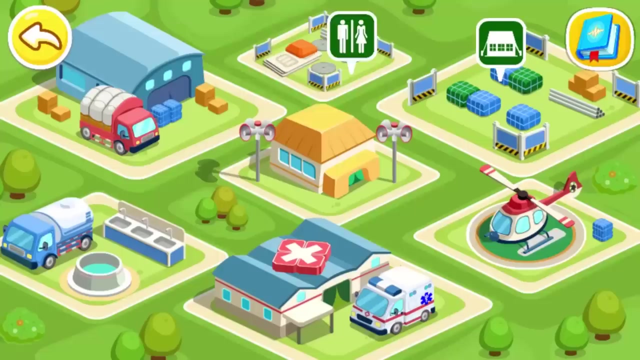 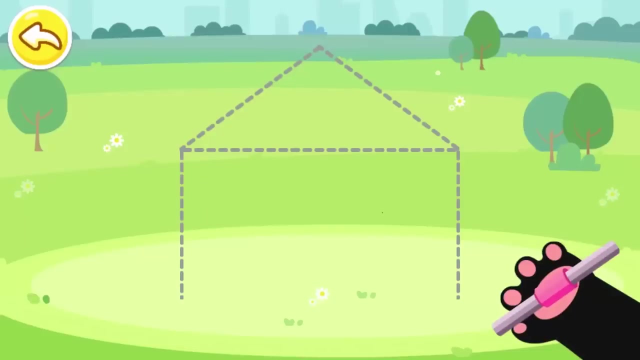 You can use this emergency toilet. What is the sign for the emergency toilet? You can use this emergency toilet. Wow, an emergency toilet has been built. Emergency shelter To pitch a tent. we need to set up poles. Where should I put this pole? 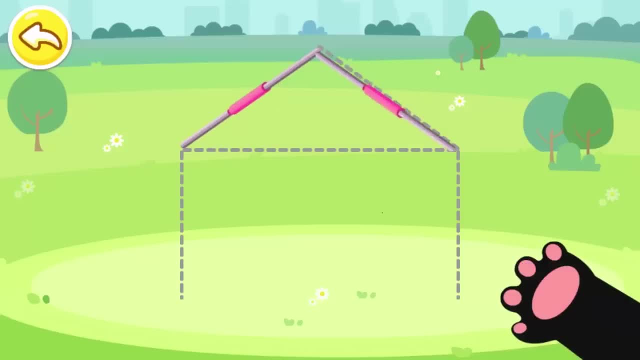 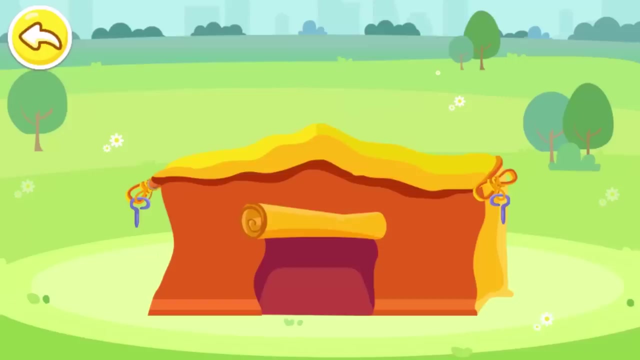 One, Two, Three, Four, Five, Great. All the poles are up, Cover them with the tent, Like this Emergency. The tent has blown down in the wind. To secure the tent we need to fasten the ropes to the earth. 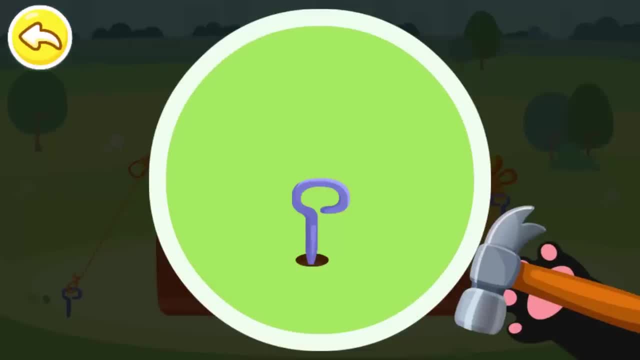 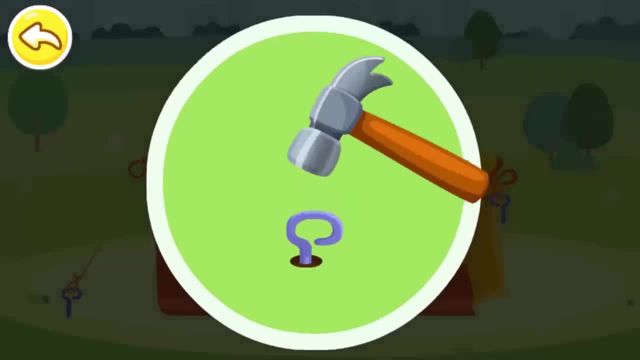 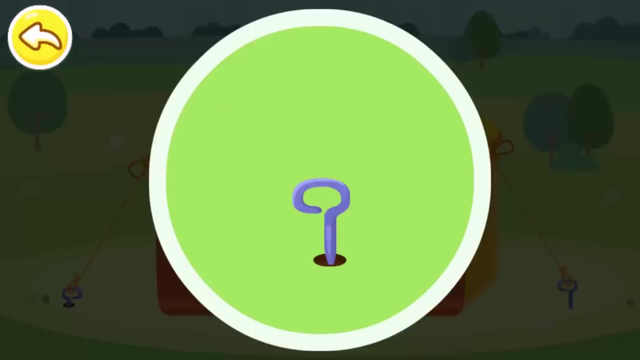 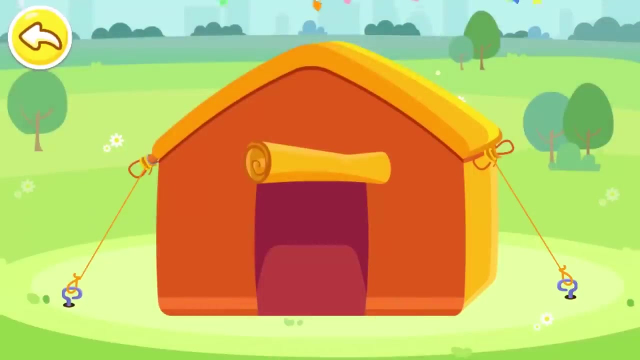 Hammer the nail and then tie the rope to it. Three, One, two, three, four. One side is fixed. Now let's do the next one: One, two, three, four. Wow, The tent is set up, Awesome. 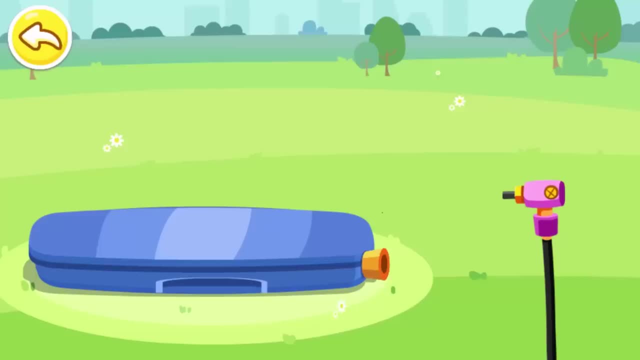 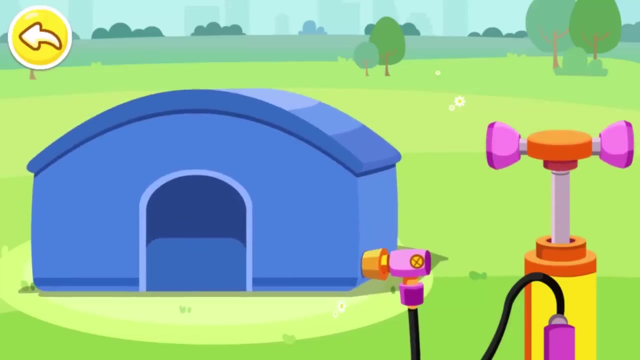 We need to set up another air tent. You need to attach the air pump to the inlet. What can happen if we blow air inside the tent? One, two, three, four, five, Wow, The tent is set up. Awesome. 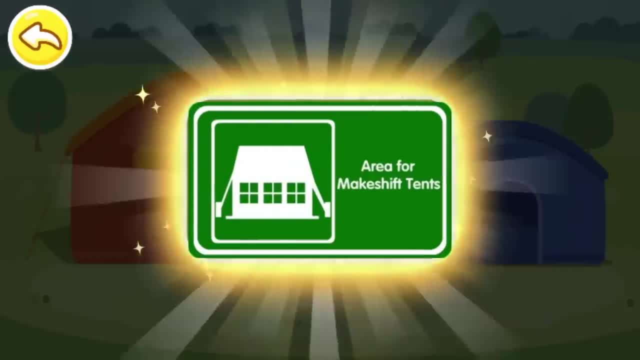 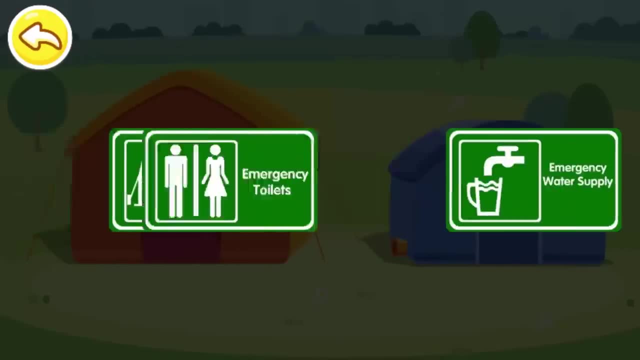 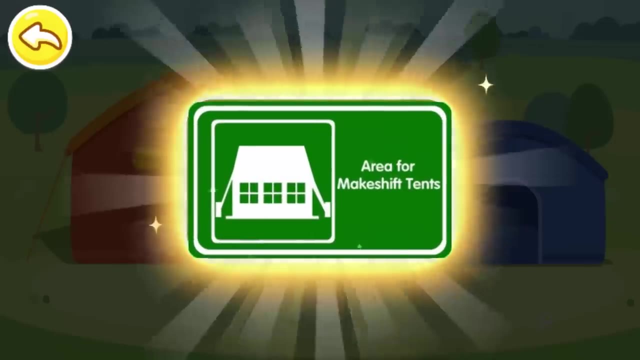 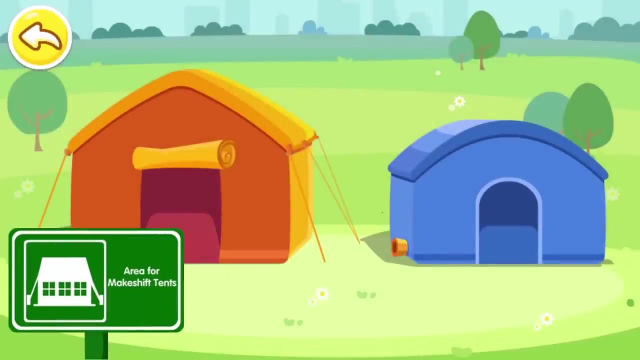 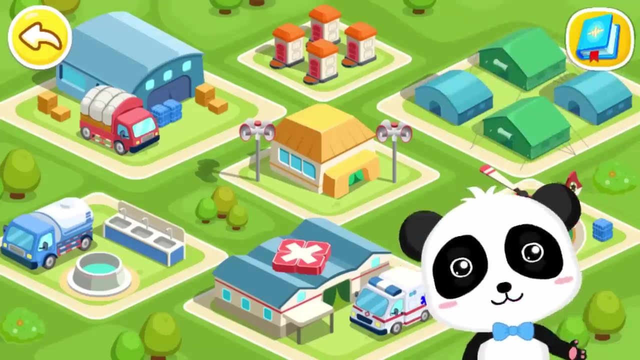 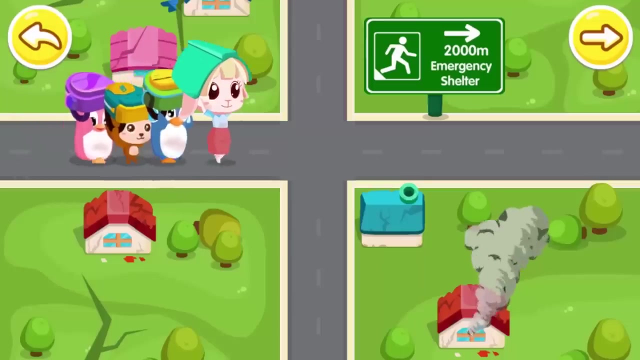 Here is the emergency shelter. You can come and sleep here. Do you know the sign for an emergency center? That's right, It's the sign for the emergency shelter. Yay, We finished building an emergency center. Follow the sign and you can find an emergency shelter. 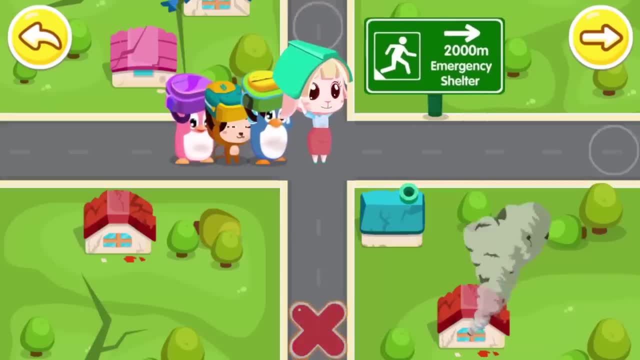 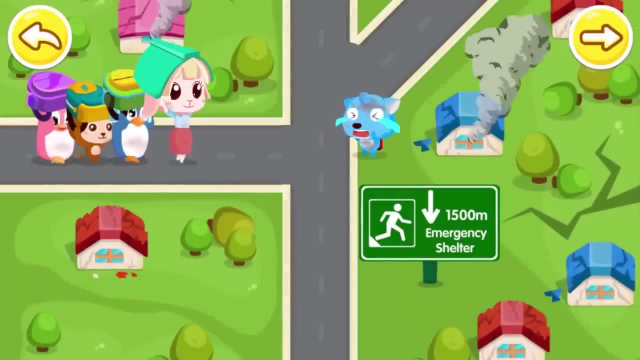 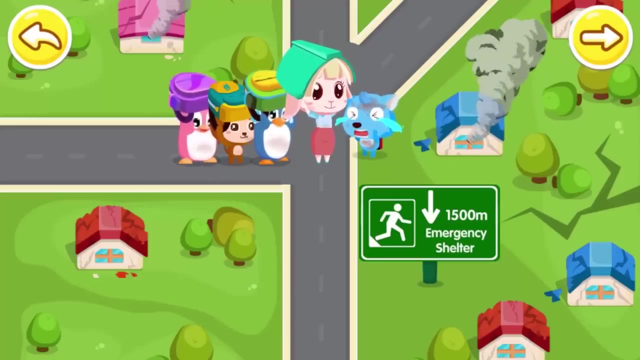 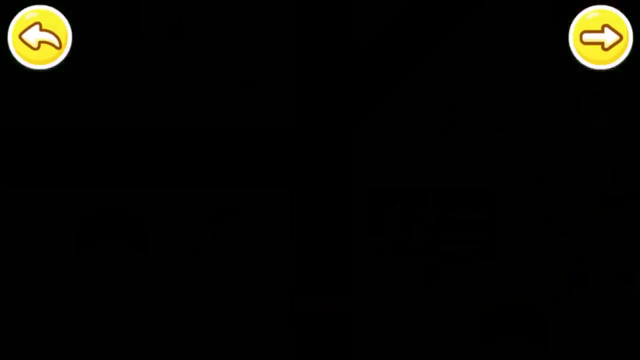 That's not the way to the emergency shelter. Aha, This is the way. Oh no, I cannot find the directions to the emergency shelter. Follow us, we will take you to the emergency shelter. Yes, thank you. Yes, it's the right direction. How can I get to the emergency shelter? 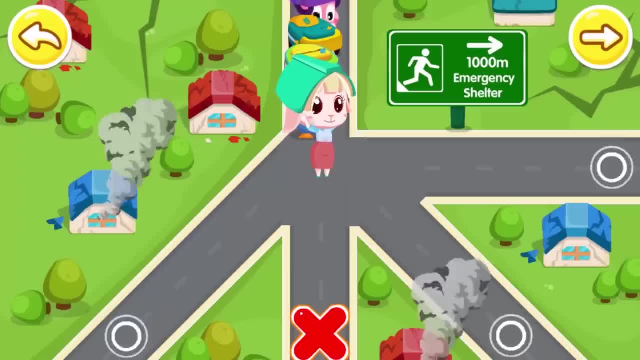 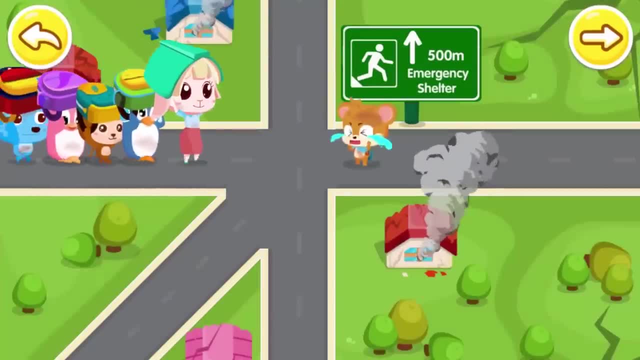 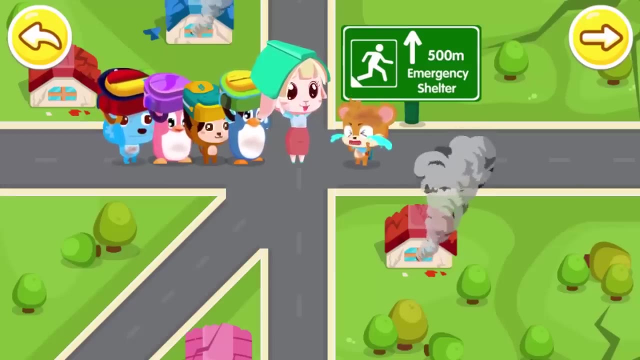 It's wrong. check the direction of the sign again. Aha, This is the way. Oh, I have no idea how to get to the emergency shelter. Follow us, we will take you to the emergency shelter. Alright, thanks, Yes, it's the right direction. 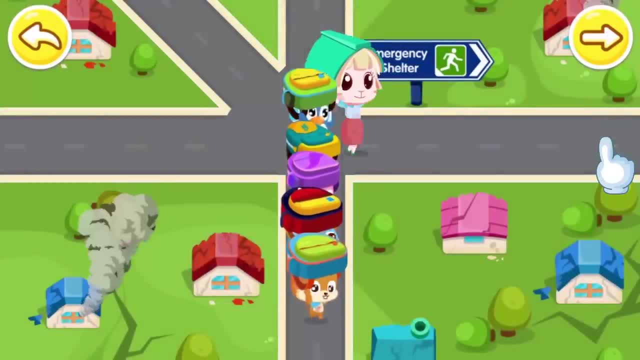 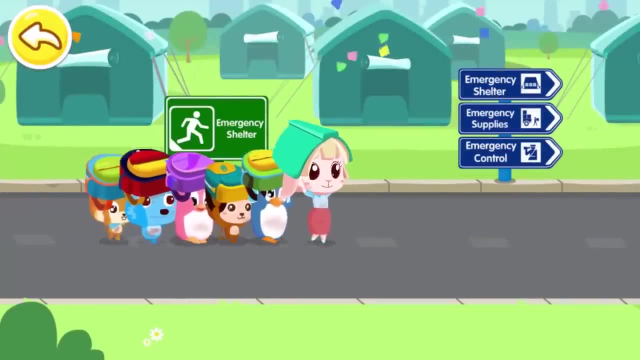 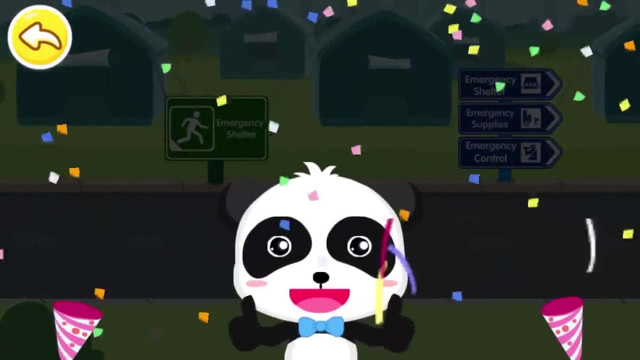 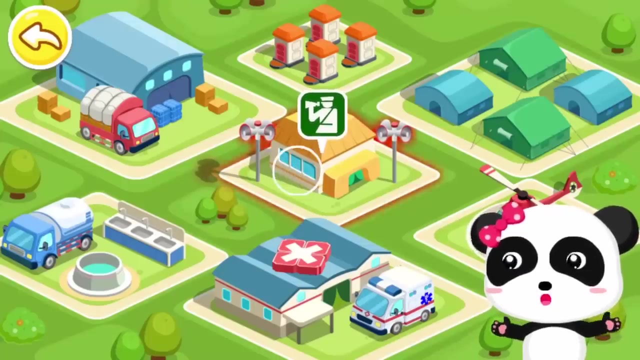 Which way should I go? Aha, This is the way. Aha, This is the way. Wow, Thanks to you, I was able to get to the emergency shelter. You need to register before you can go to an emergency shelter. Where should I go to register? 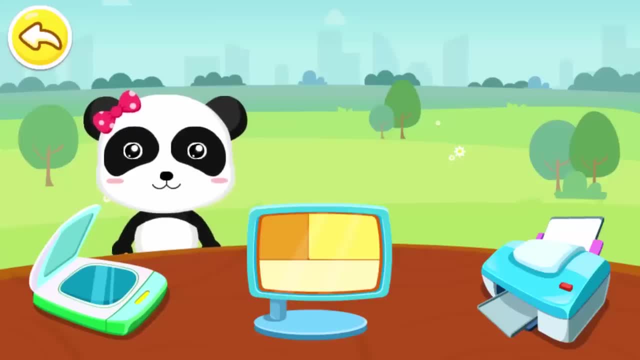 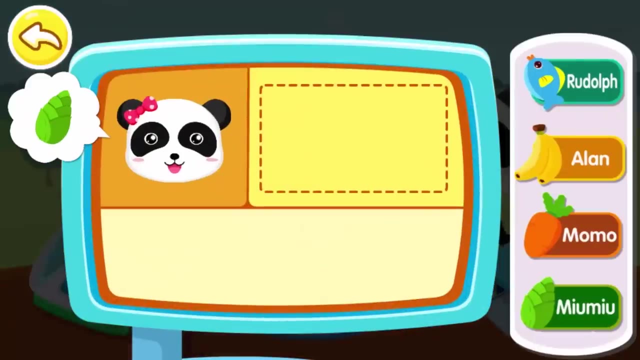 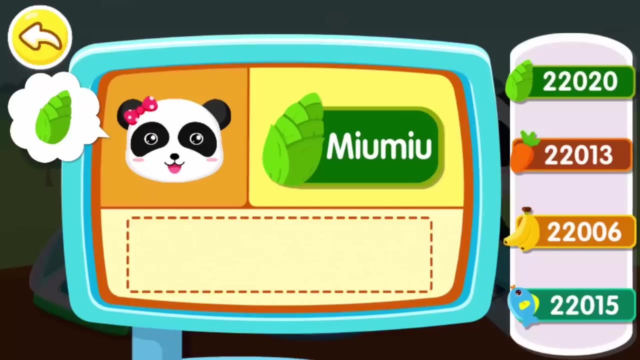 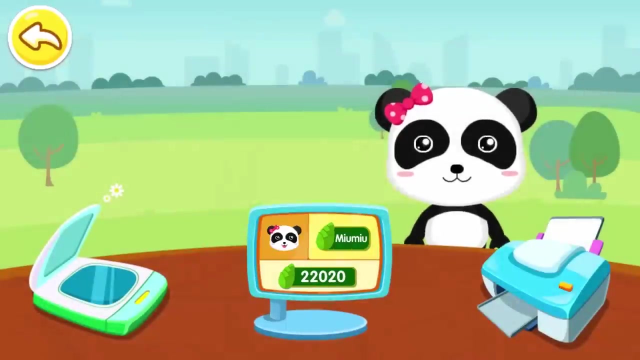 Emergency Control Center. Please show me your ID. Here is my ID card. Great, I'll make a scanned copy. My name is Miu Miu. Can you find my name? My number is 22020. Registration is all done. Here is your ID back. Wow. 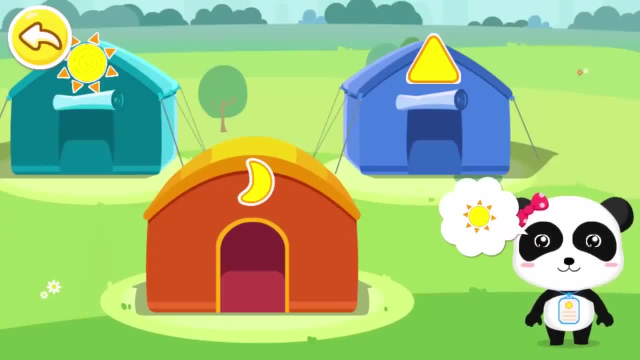 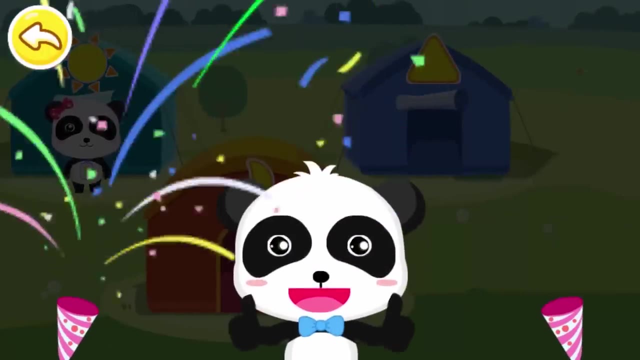 I'm so lucky. Oh, thanks, Help me find the right tent. No, that's not my shelter. He was wrong. You need to register before you can go to an emergency shelter. You need to register before you can go to an emergency shelter. Fire, Fire, Rush out firefighters. 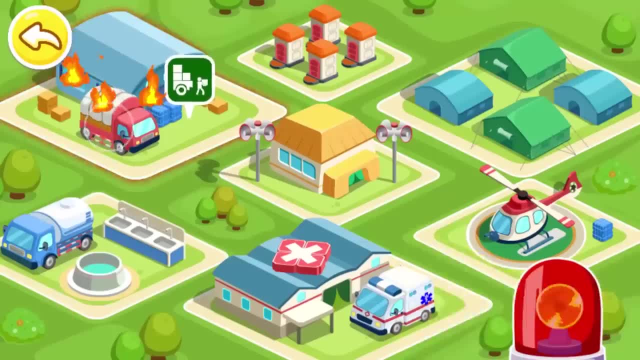 Emergency supplies. Do you know how to use the fire extinguisher? Do you know how to use the fire extinguisher? You can bring some fire extinguishers. You can bring some fire extinguishers. Extinguisher: first, pull the pin in the handle. 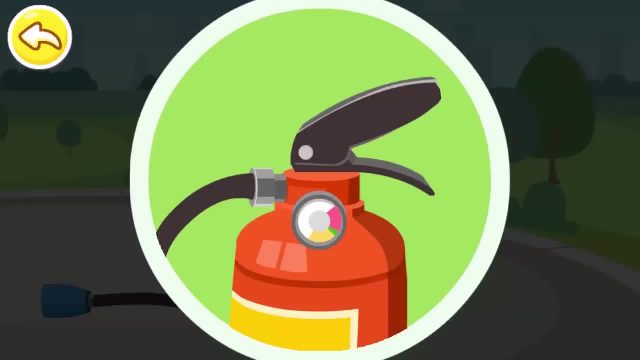 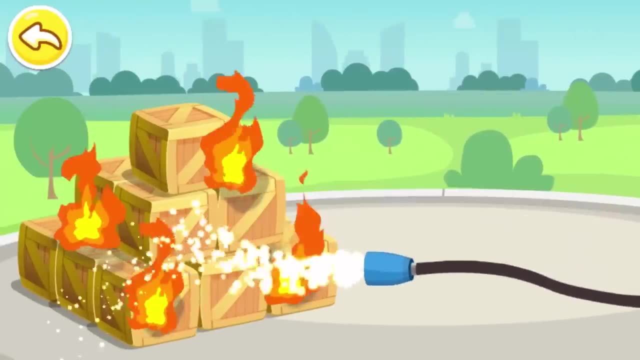 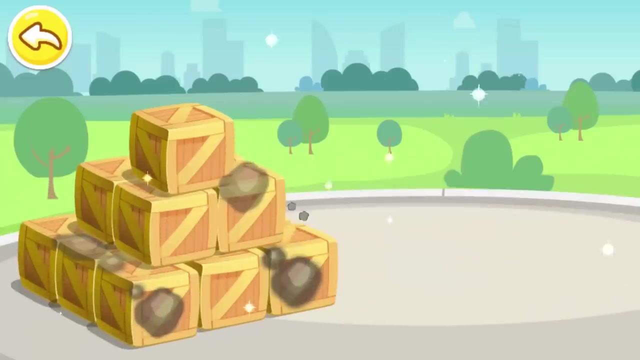 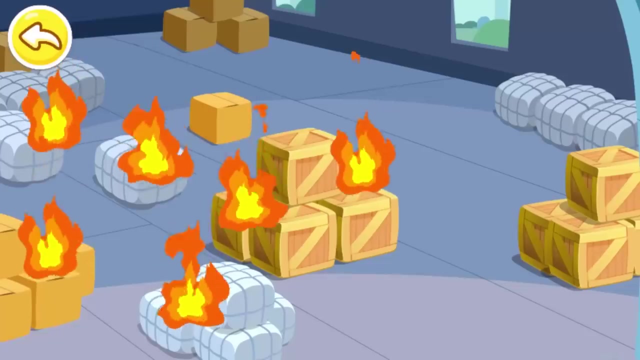 Secondly, grip the handle. Thirdly, aim the nozzle at the base of the fire. Great, Extinguish the fire right away. Uh-oh, we need the fire hydrant to extinguish a fire. Step one: open the hydrant. 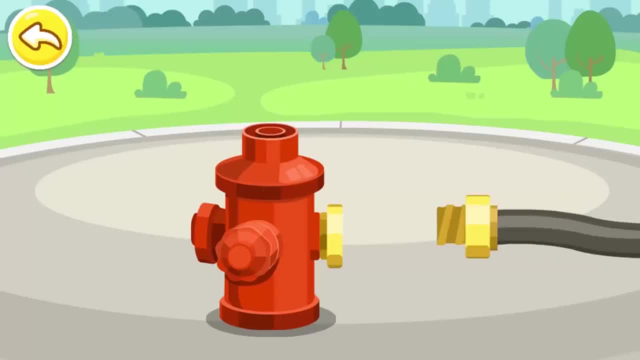 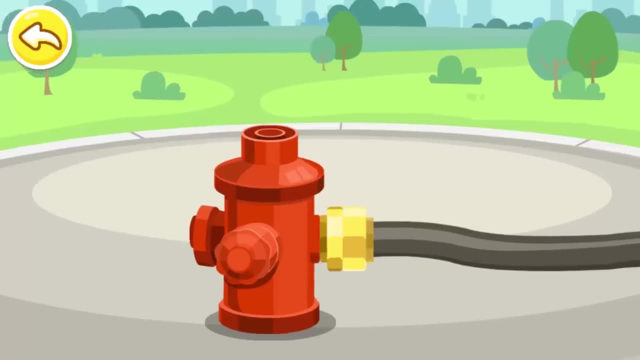 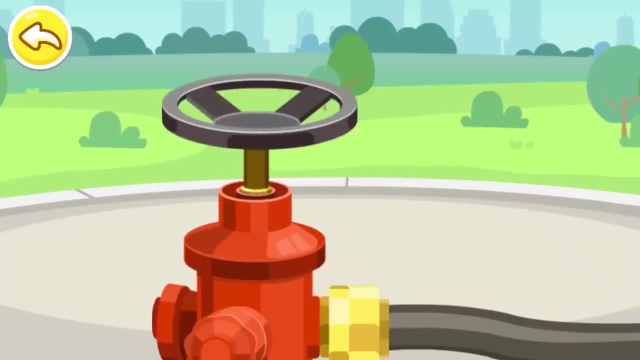 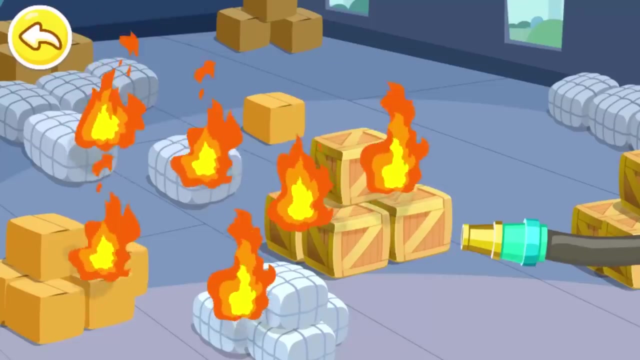 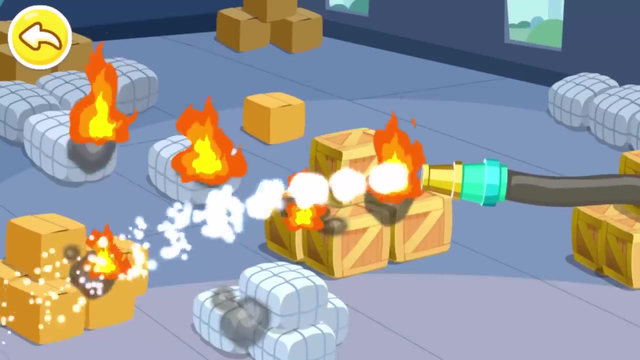 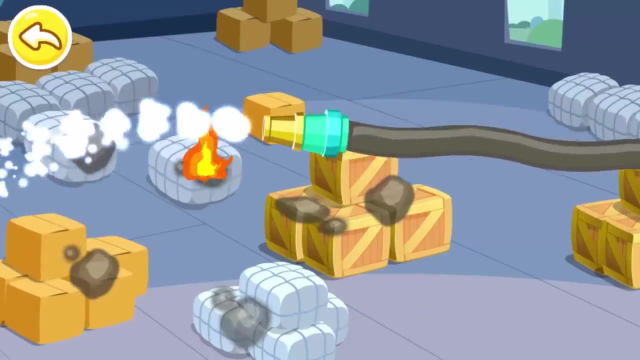 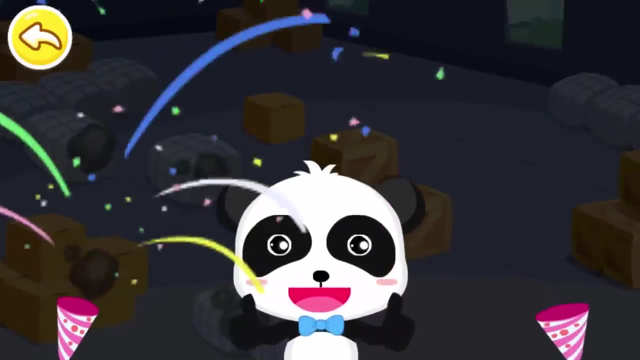 Step two: connect the hydrant hose and fasten the joint. Step three: set up the valve And turn it. Step four: spray it on the fire. Guys, fire is so dangerous that you shouldn't play with it. I'm so hungry. Where can I get some food? 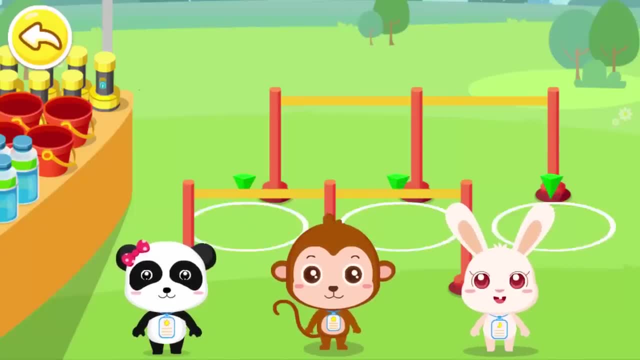 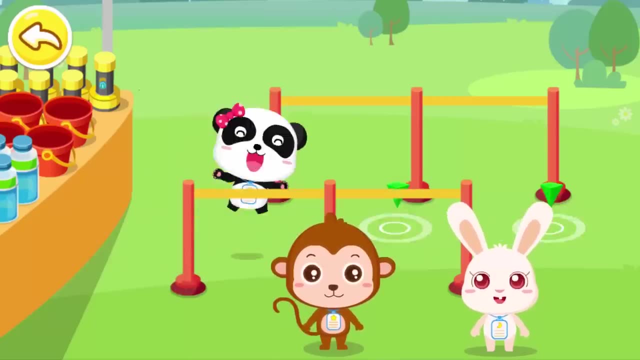 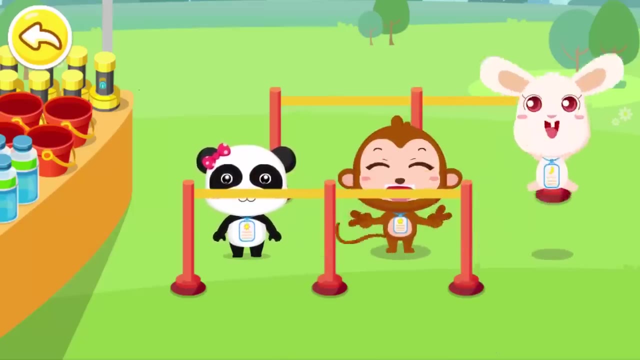 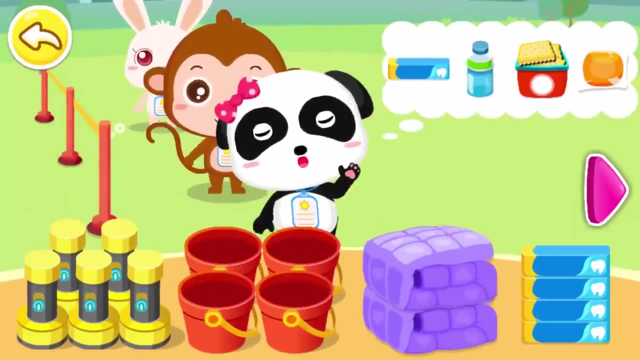 Emergency supplies. You should queue up when you receive goods. Can you make people queue up? Thanks, Thanks, Thank you. I need these things. Can you help me find them? Water bottle: No, that's not what I need. Toothpaste. 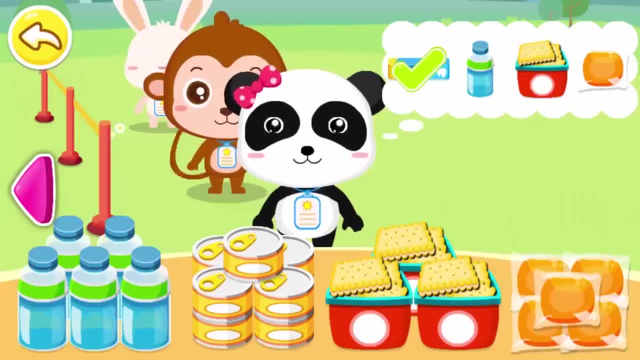 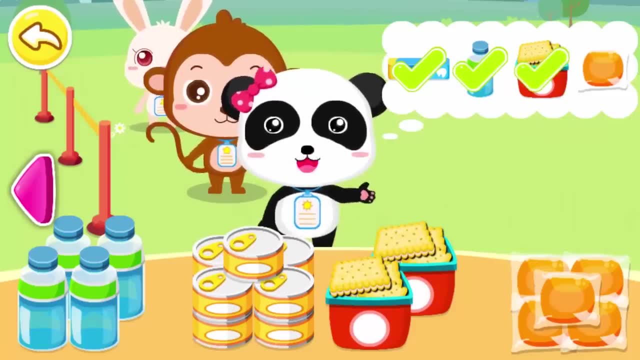 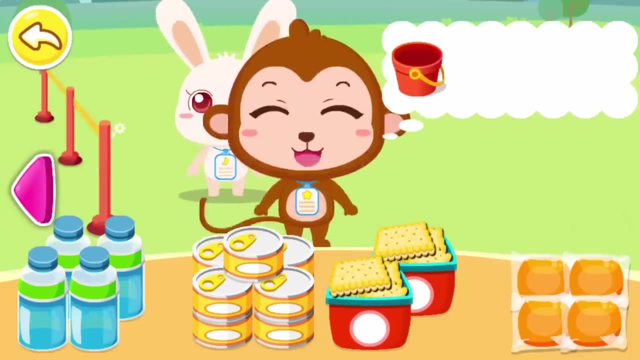 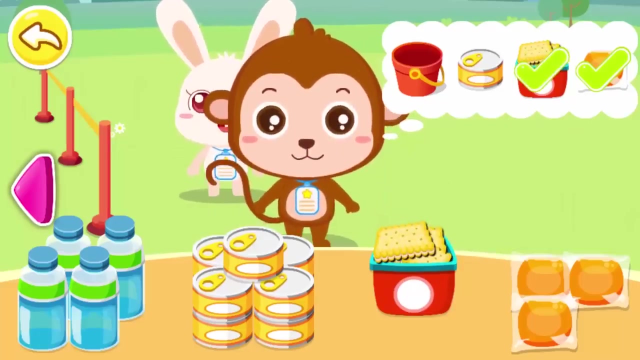 Yes, exactly Water, Thanks. Cookies: Yes, exactly Bread, Thanks. Wow, I found everything. Thank you, I need this stuff. Can you help me find it? Bread: Yes, exactly Cookies, Cookies, Thanks. 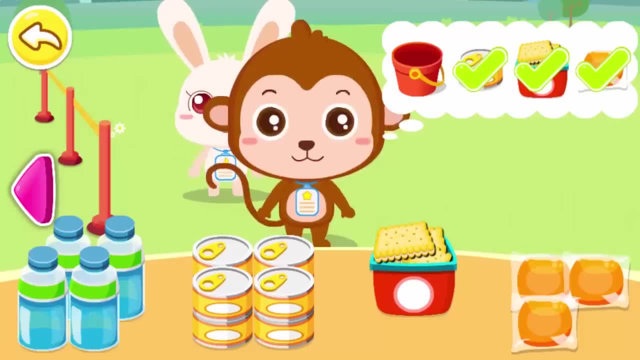 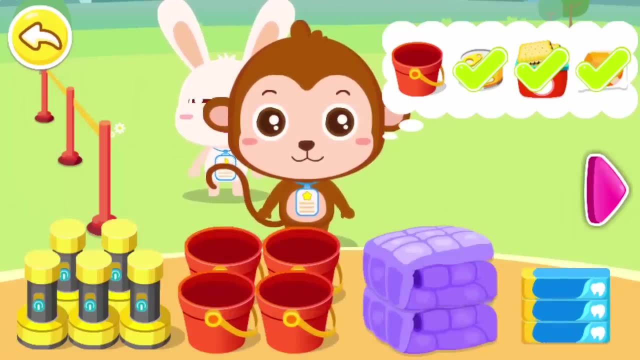 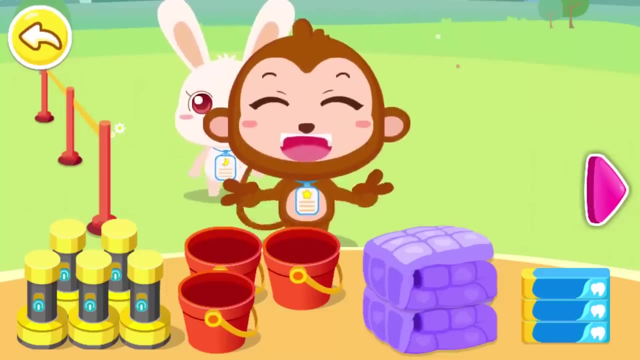 Canned food: Yes, exactly. Water- No, that's not what I need. Water- No, that's not what I need. Water Water: Yes, exactly. Thanks, Wow, I found everything. Thank you, I need these things. Can you help me find them? 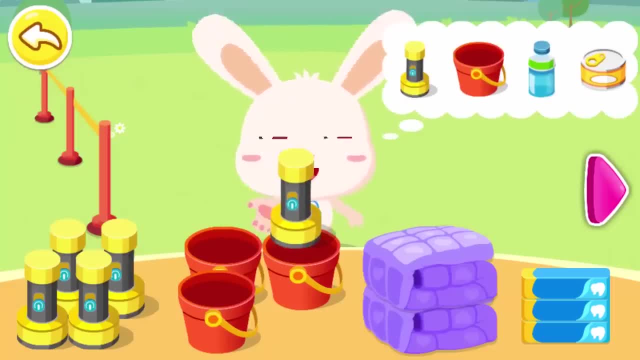 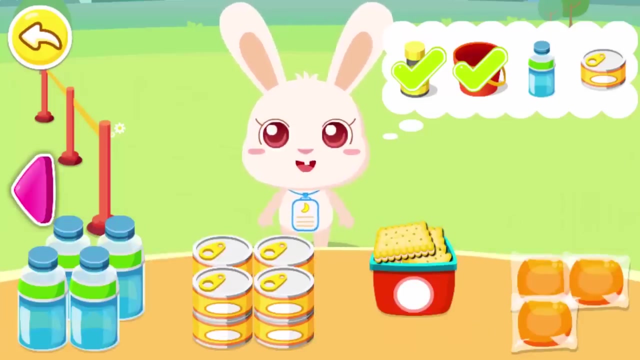 I need these things. Can you help me find them? Flashlight: Yes, exactly. Water bottle, Thank you. Well, No, that's not what I need. Well Water: Yes, exactly Canned food, Thank you. 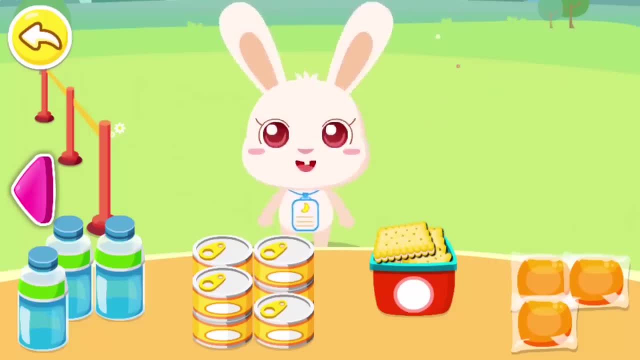 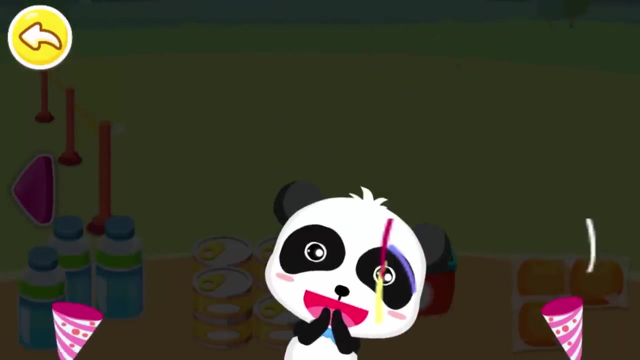 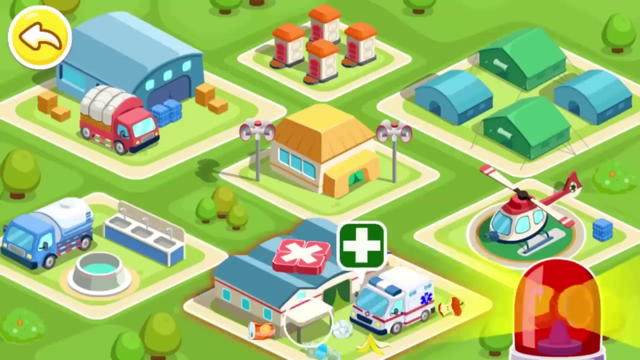 Wow, I found everything. Thank you, Wow. thanks to your help, everyone gets emergency supplies. You can get food and household goods at the Emergency Supply Center. Oh, there is too much rubbish here. We need to clean it up. Emergency medical treatment. 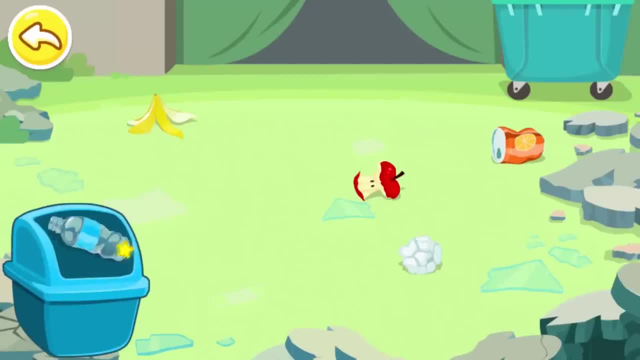 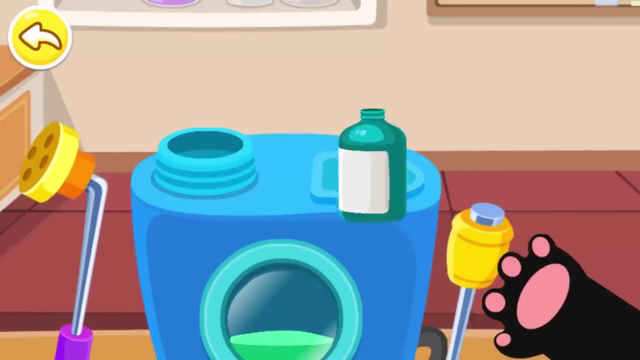 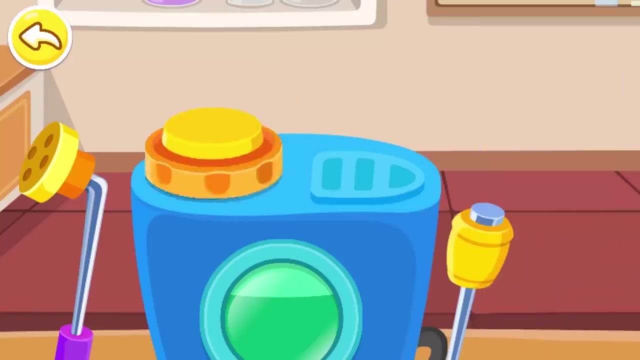 Throw the trash into the trash can. Don't just throw trash anywhere. Oh, there are mosquitoes in the trash. Please catch them. First, spray the insecticide. Secondly, cover it. Thirdly, press the button on the insecticide tool. 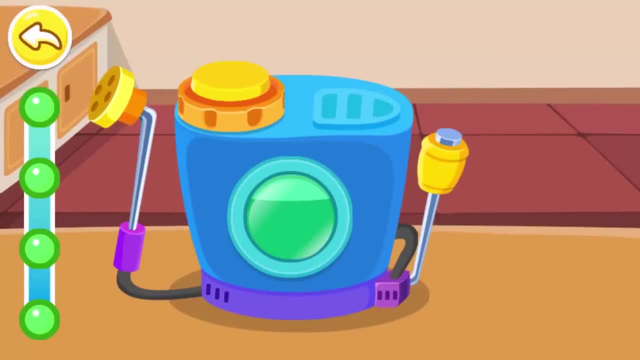 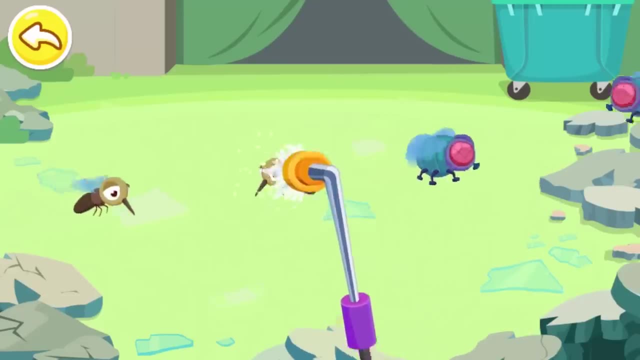 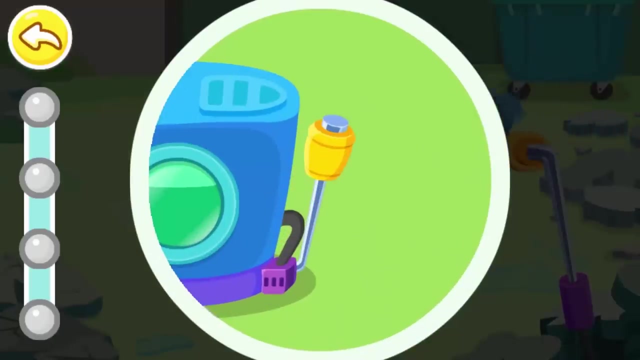 Now, let's get rid of all the mosquitoes. Now, let's get rid of all the mosquitoes. Now, let's get rid of all the mosquitoes. Uh-oh, we need more pressure. Uh-oh, we need more pressure on the insecticide tool. 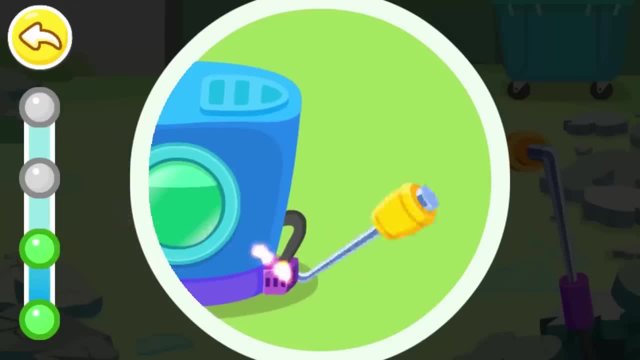 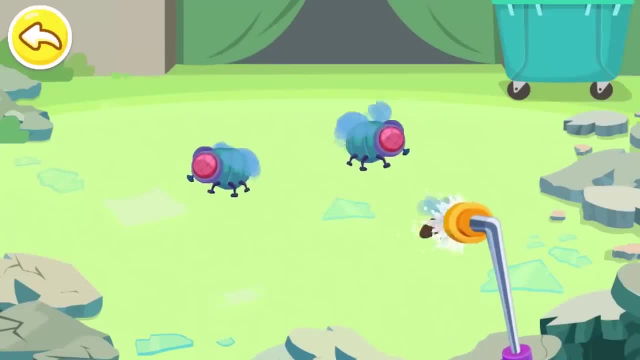 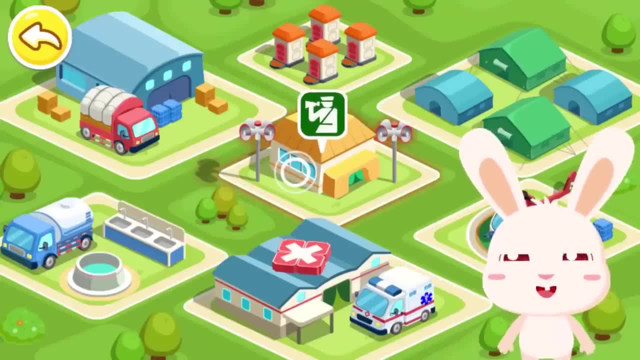 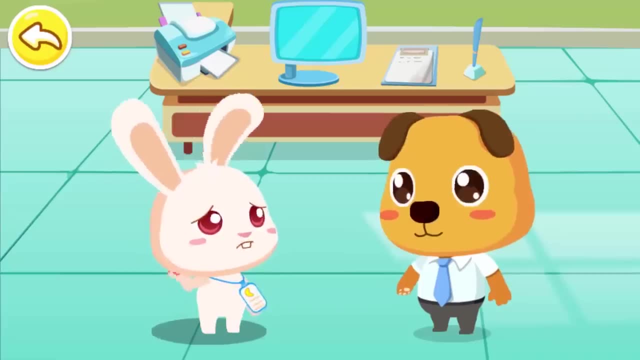 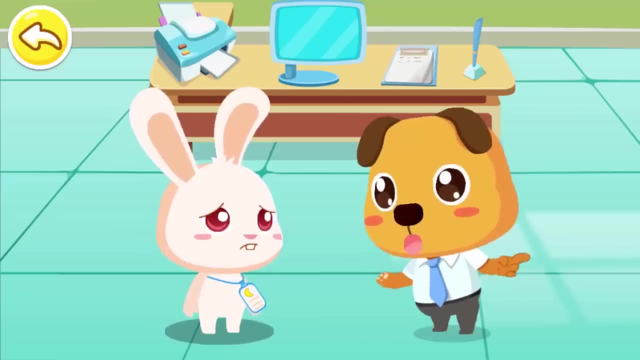 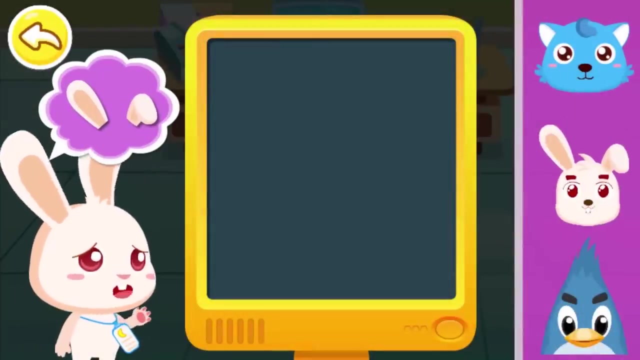 Wha. Where's my dad? What should I do? Emergency Control Center. Where is my dad? Emergency Control Center. Emergency Control Center. Don't worry, can you describe what your dad looks like? My dad has long ears. My dad has long ears. 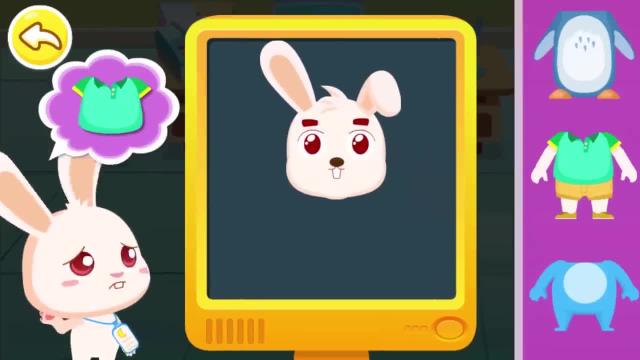 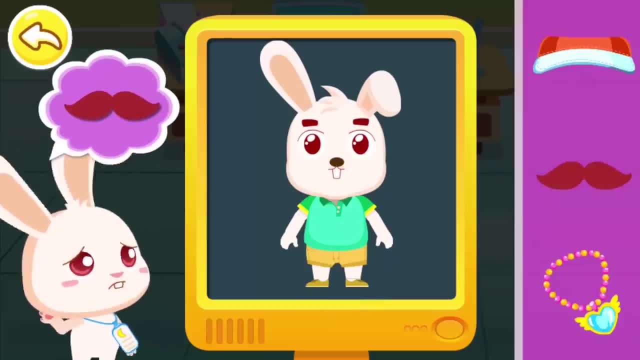 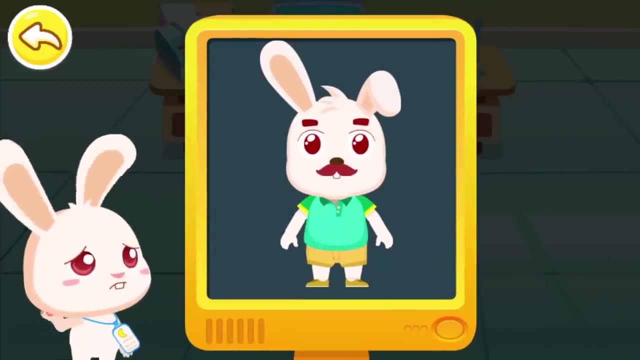 My dad has long ears. My dad wears green clothes. My dad wears green clothes. My dad has a thick beard. My dad has a thick beard. My dad wears a white shirt. My dad wears a white shirt. My dad wears a white shirt. 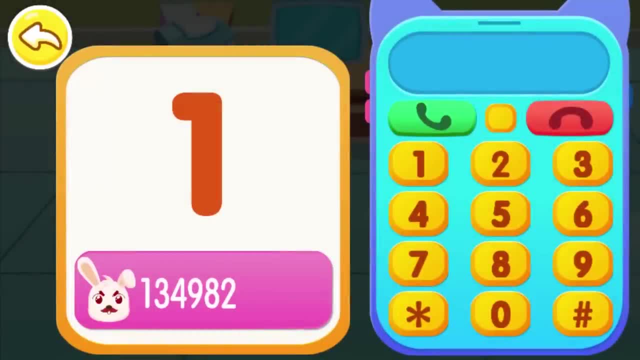 Yes, that's my dad. Yes, that's my dad. Call your dad now. 1, 3, 4, 9, 8, 2. 1, 3, 4,, 9,, 8, 2. 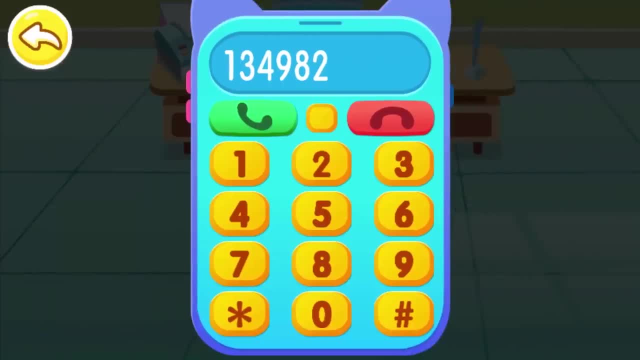 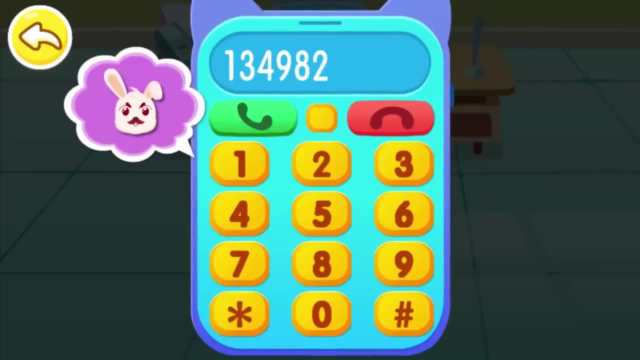 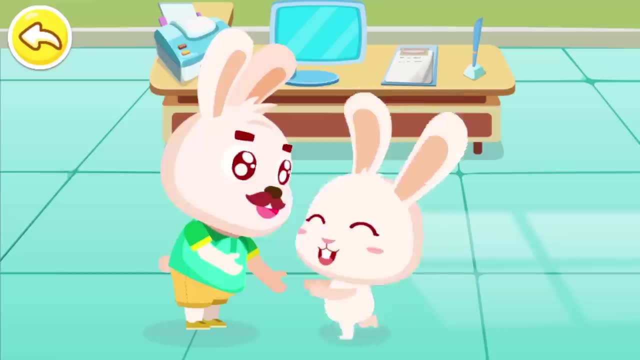 Hello, are you Momo's dad? Hello, are you Momo's dad? Momo is waiting for you at the Emergency Control Center. control center. momo, you shouldn't go alone without your dad. no, i won't go anywhere without my dad. 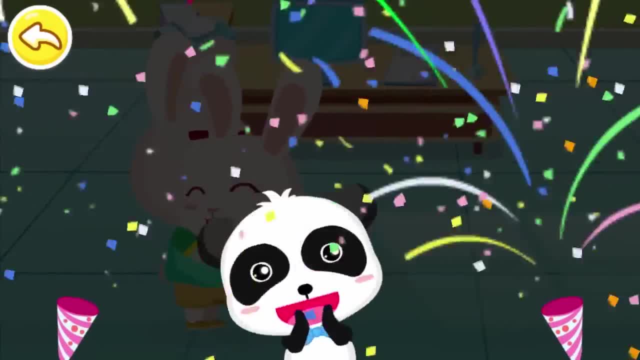 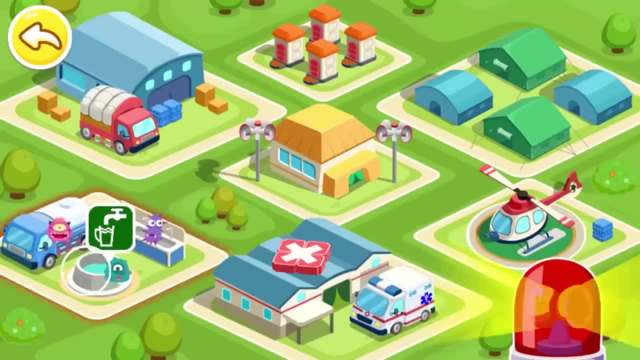 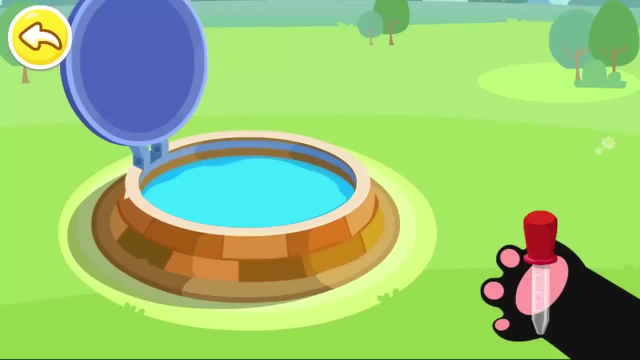 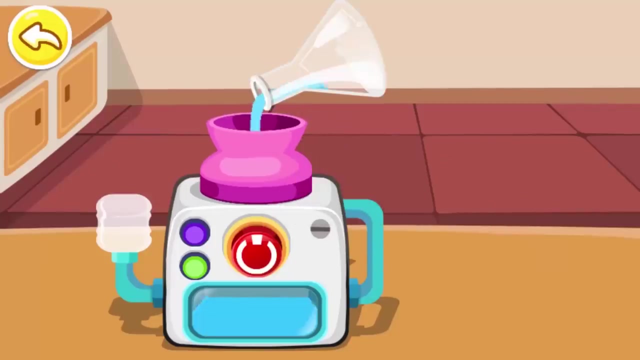 if you get lost at the emergency shelter, you can go to the emergency control center. if a disaster happens, water might be contaminated. let's go check emergency water supply. pour some water in the bottle- so great. let's go examine the water. Uh-oh, The water quality is bad. We need to disinfect it. 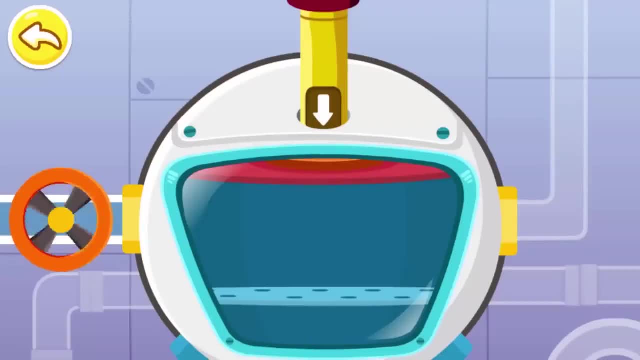 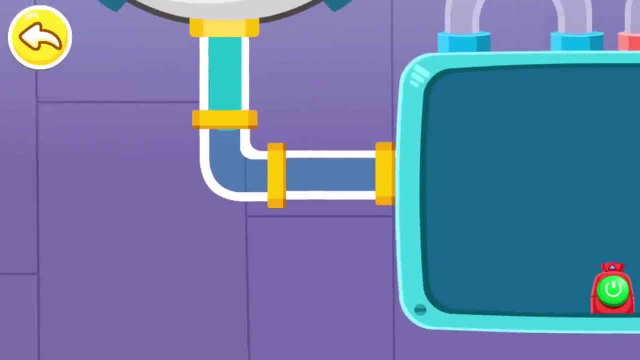 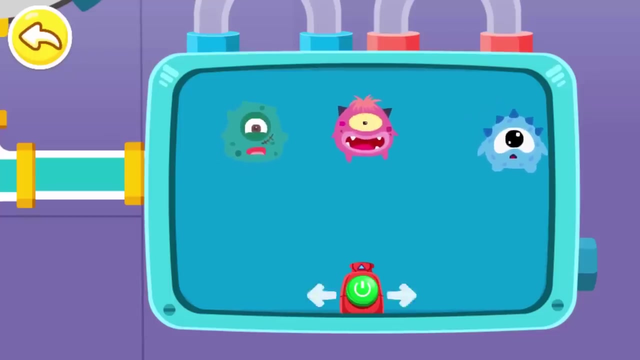 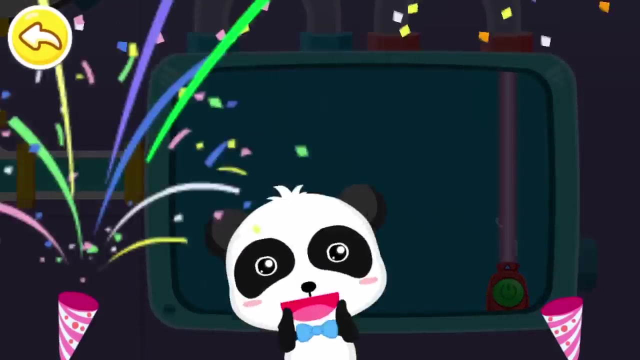 Step 1. Open the valve. Step 2. Filter out the dirt in the water. Yes, You did well. Step 3. Kill the bacteria with ultraviolet rays. Yay, All done. You can use the water right away. 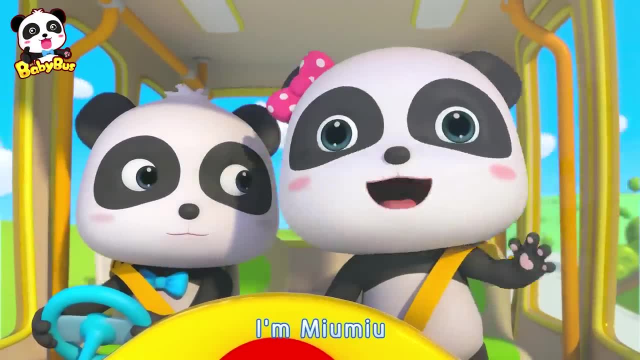 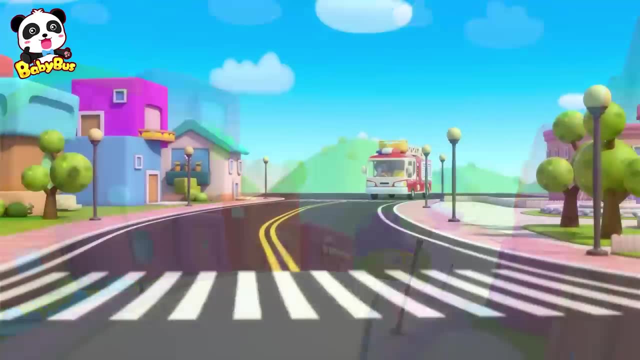 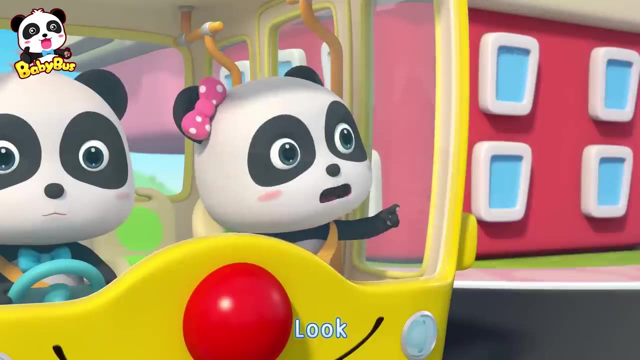 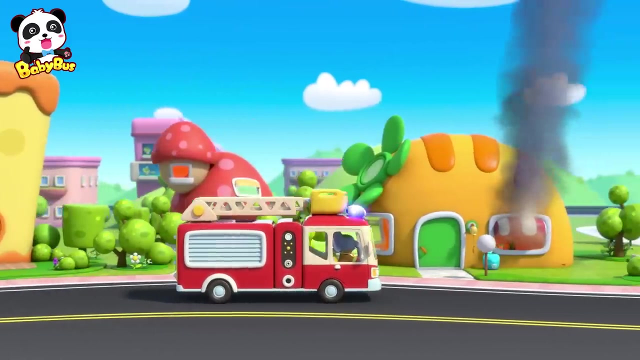 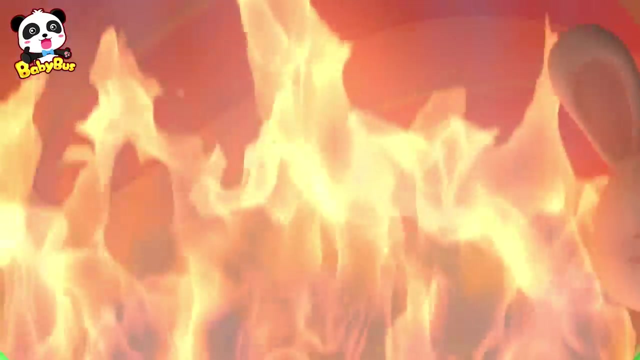 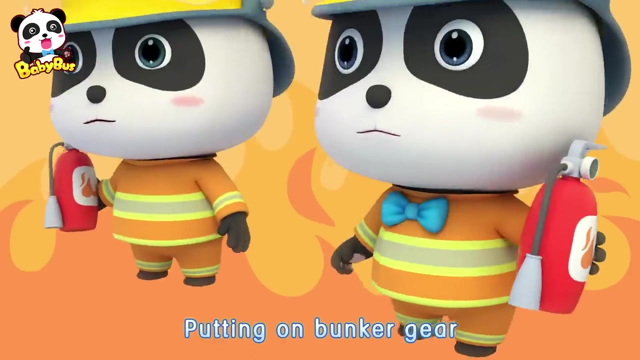 Hello, I'm Kiki, Hi Mew-mew, Wow, It's a fire engine. Look, There's a fire. Let's become firefighters and help people in danger. Firefighters, Fire, fire. Someone shout: I'm a brave firefighter. 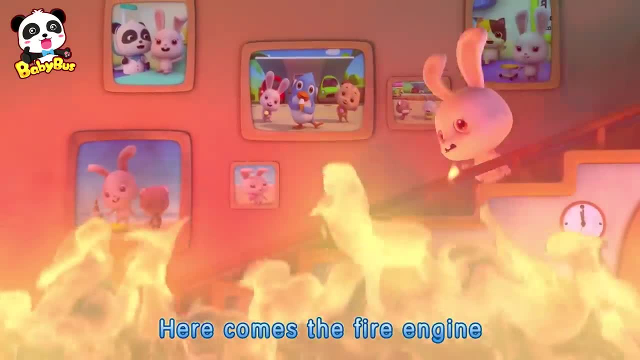 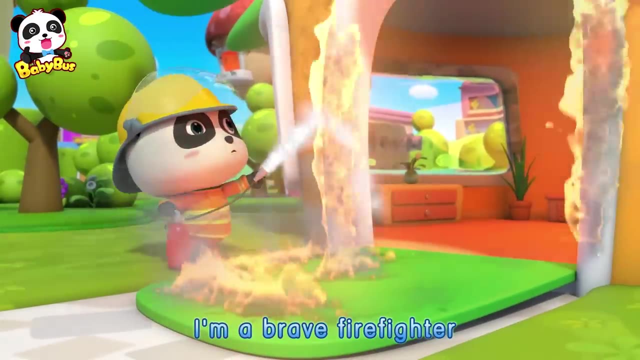 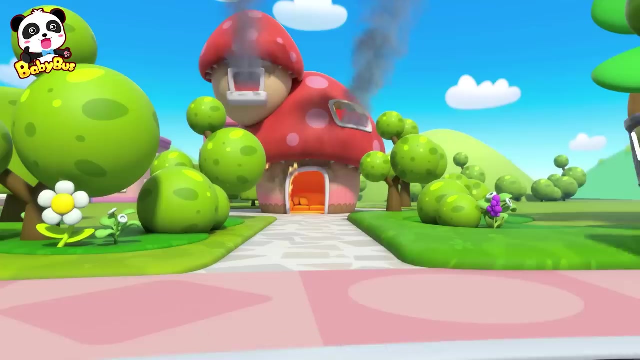 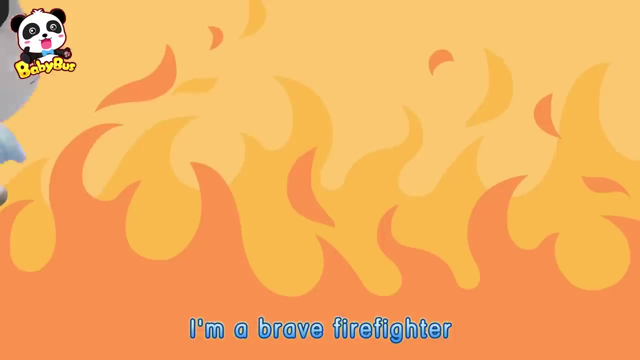 Putting on bunker gear. Here comes a fire engine. Help me, help me. Someone shout: I'm a brave firefighter. Calm down, calm down, Follow me, Let's get out of here. Fire, fire. Someone shout: I'm a brave firefighter. 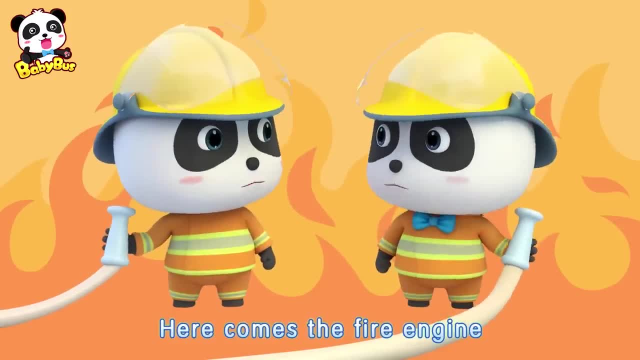 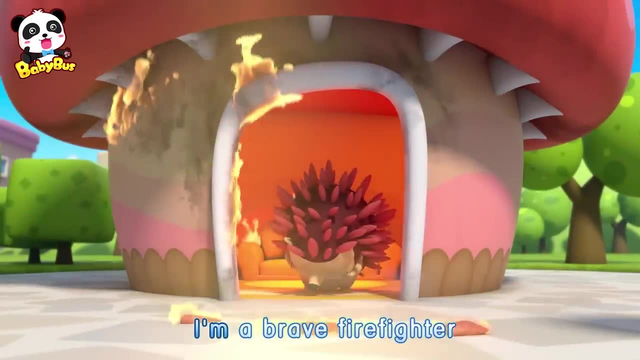 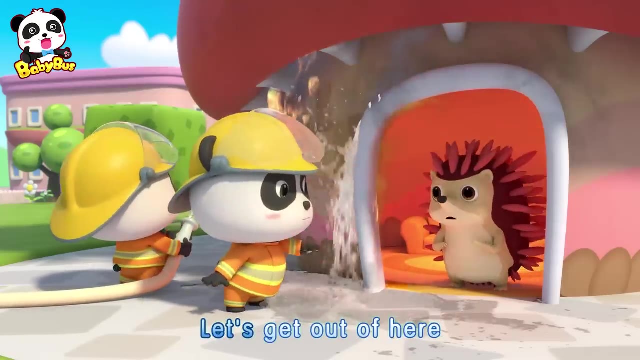 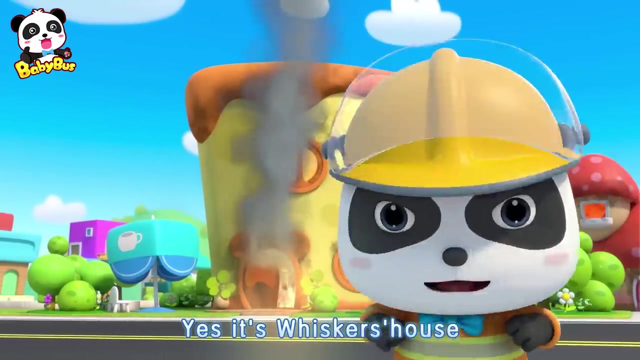 Getting a fire hose in my hand. Here comes a fire engine. Help me, help me. someone shouts: I'm a brave firefighter, Calm down, calm down, follow me, Let's get out of here. Can you see whose house is on fire? Yes, it's Whiskers' house. Let's go save him. 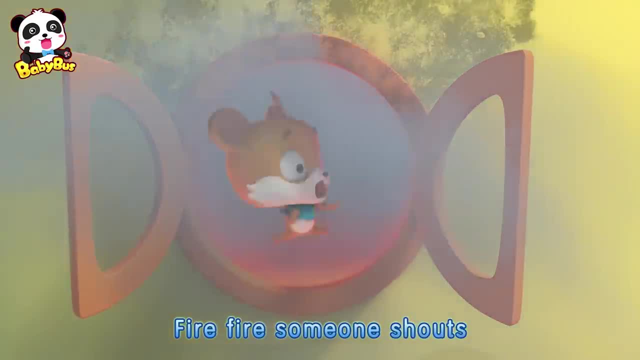 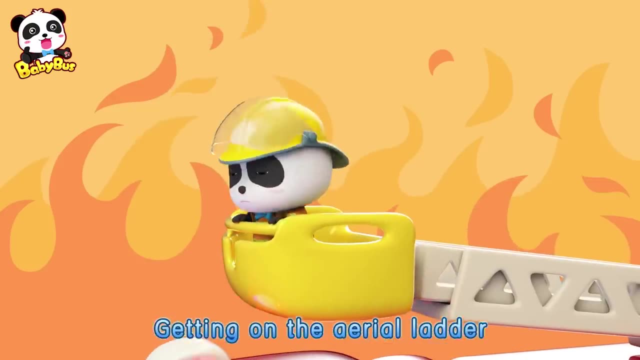 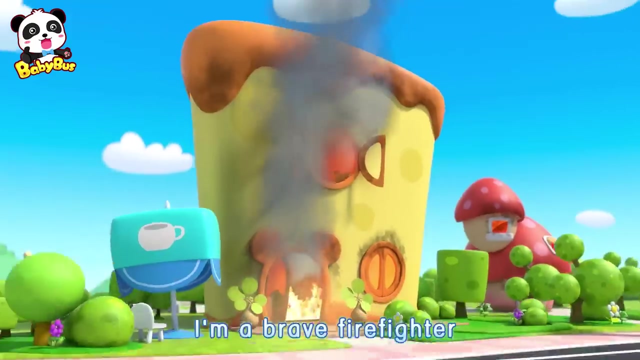 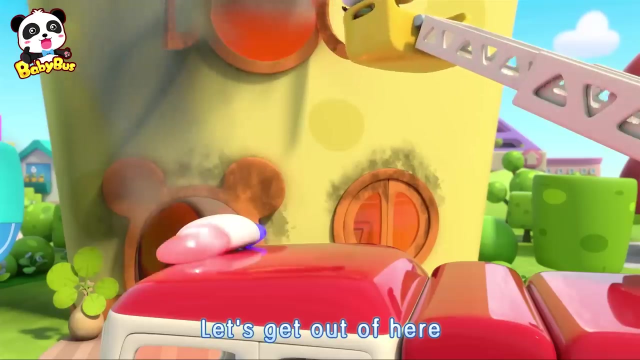 Fire, fire. someone shouts: I'm a brave firefighter Getting on the aerial ladder. Here comes a fire engine. Help me, help me. someone shouts: I'm a brave firefighter, Calm down, calm down, follow me, Let's get out of here, Help me, help me. someone shouts: 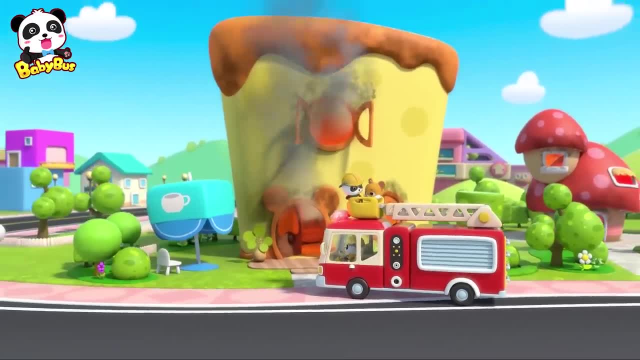 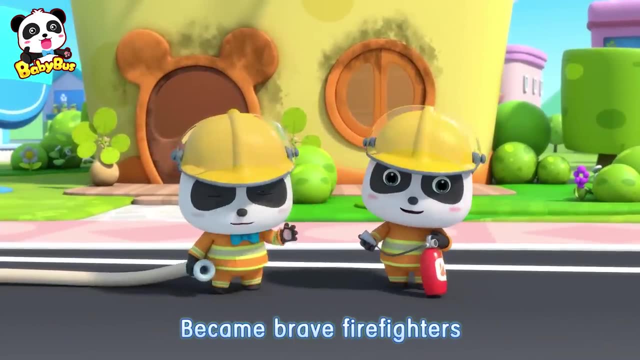 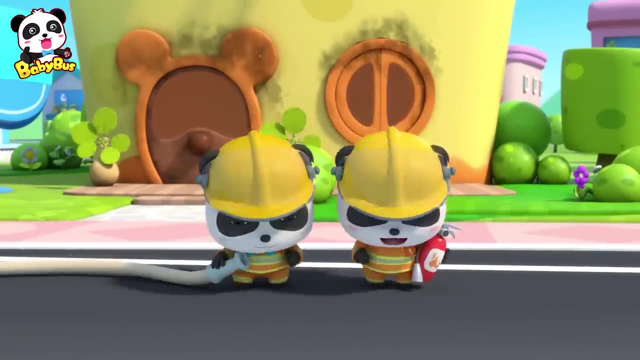 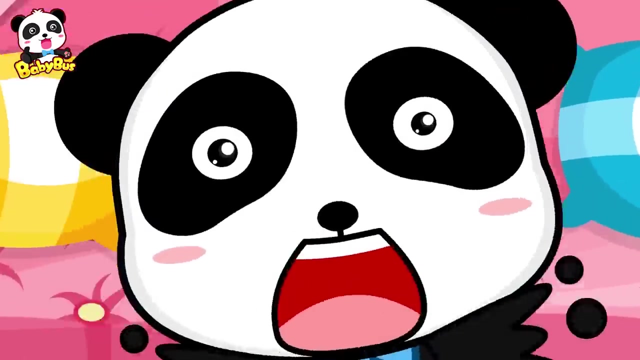 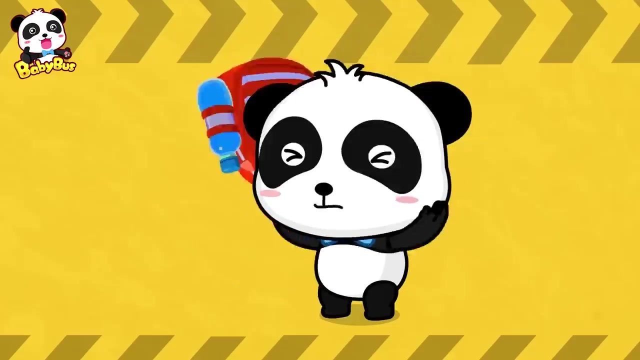 I'm a brave firefighter. Calm down, calm down, follow me, Let's get out of here. Wow, Today, Kiki and Miu Miu became brave firefighters. Let's give them medals. Yay, We won. You don't think this will be easy, right. 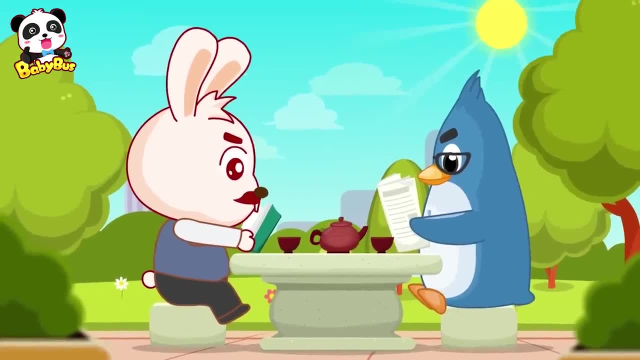 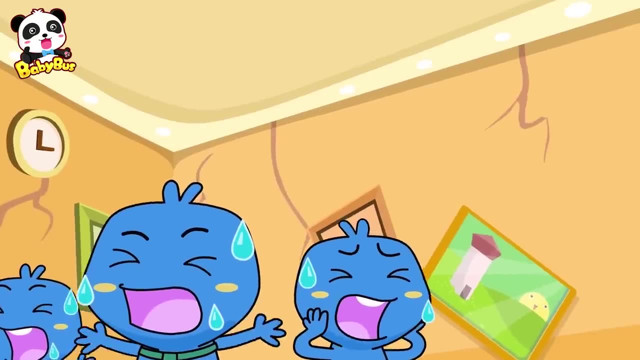 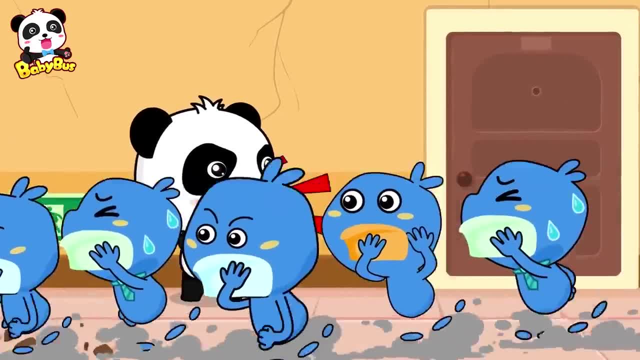 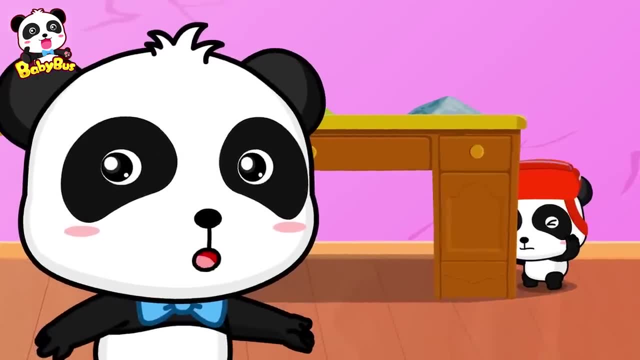 Help me, help me. someone shouts: I'm a brave firefighter, Calm down, calm down, follow me, Let's get out of here. Can you see whose house is on fire? Here comes a fire engine. Help me, help me. someone shouts Under the bed. 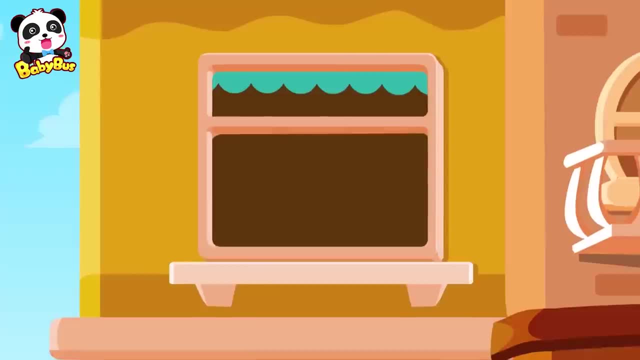 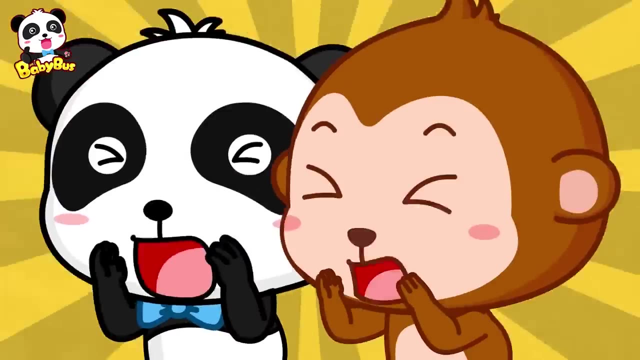 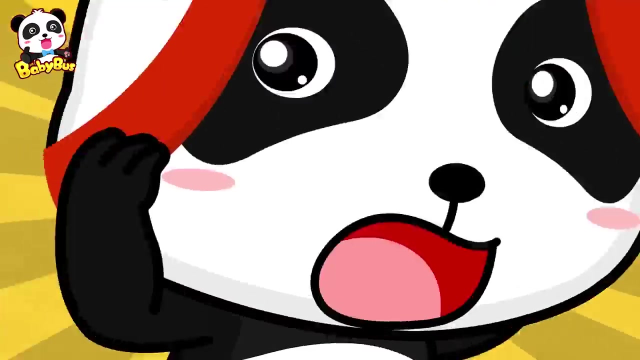 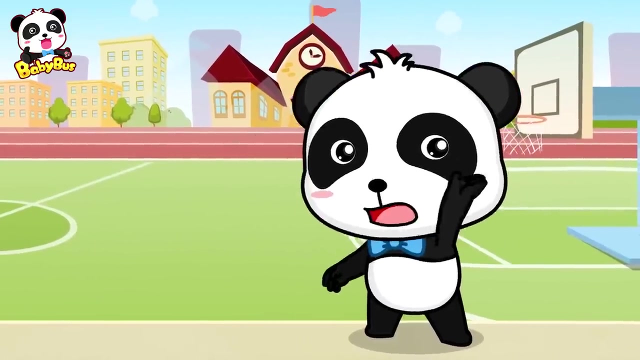 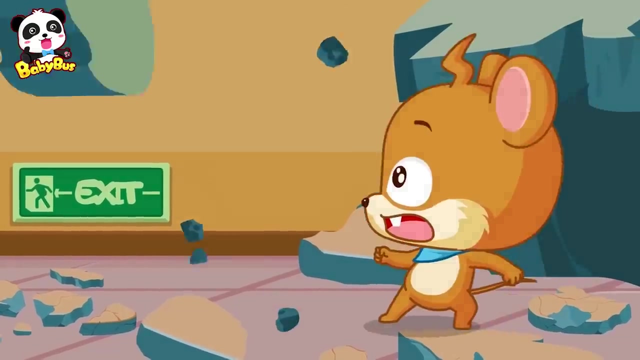 Don't use elevator, Take the spare, Do not panic And be prepared. Earthquake, Earthquake, Earthquake. Don't panic, Take cover, Go hide Outside. Don't you open ground? Don't be, Don't look around. If you're trapped, Stay calm, Keep your strength. 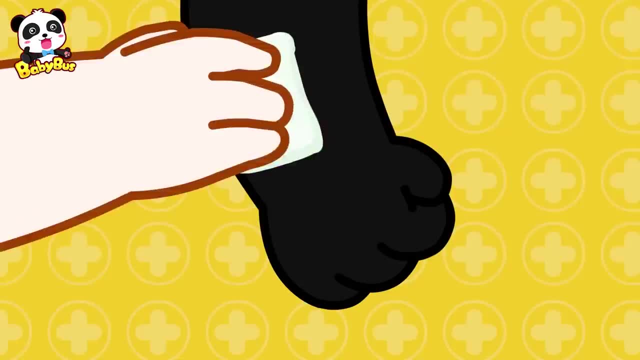 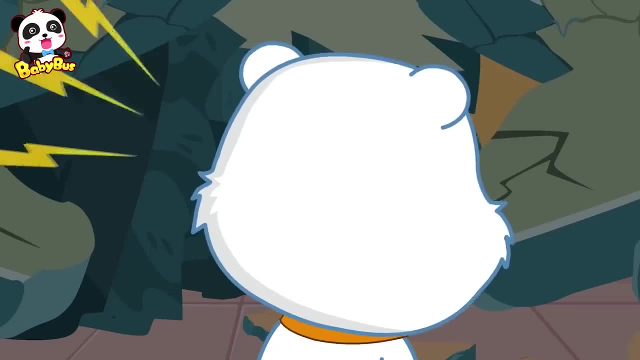 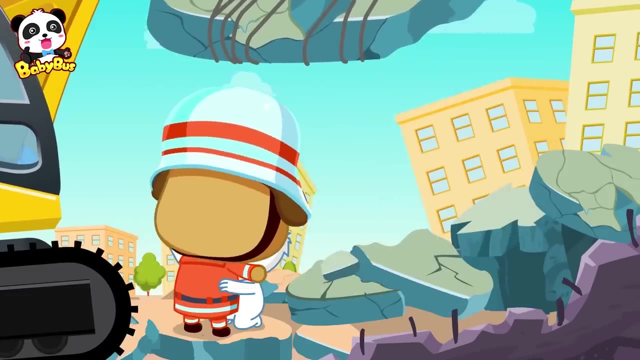 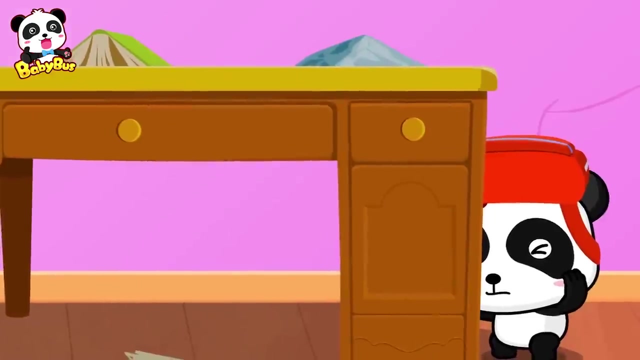 Don't make a sound. If you're bleeding The stone hard, Treat your wound With cotton wrap. When you hear people You can shout. Keep in mind The help will come. Sober mouth. Don't send your head. Hide your Body under the desk. Don't use elevator. Take the spare. 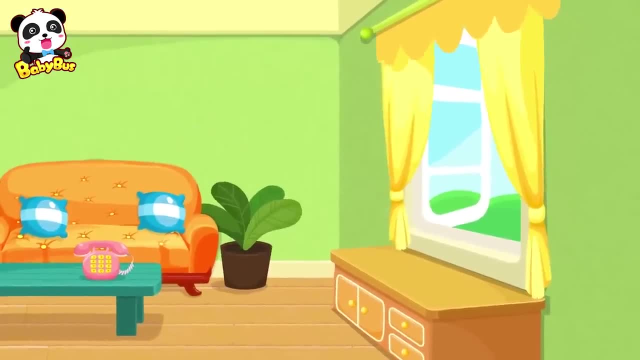 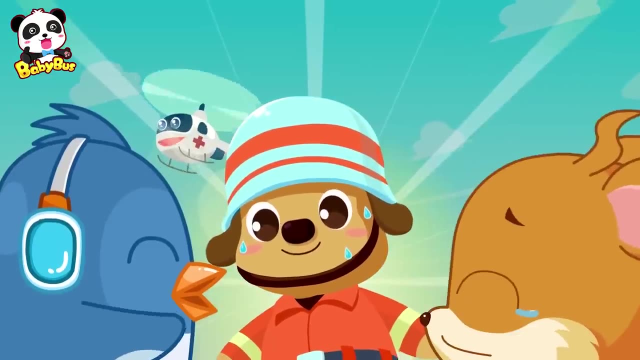 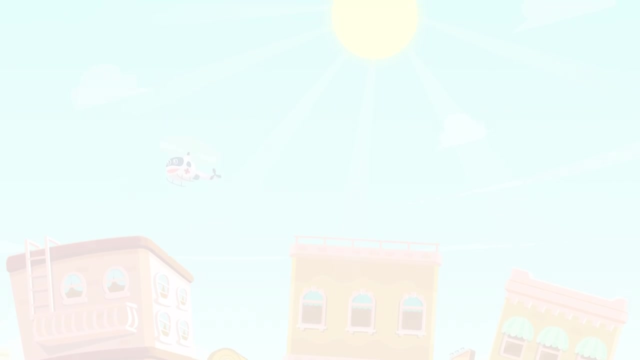 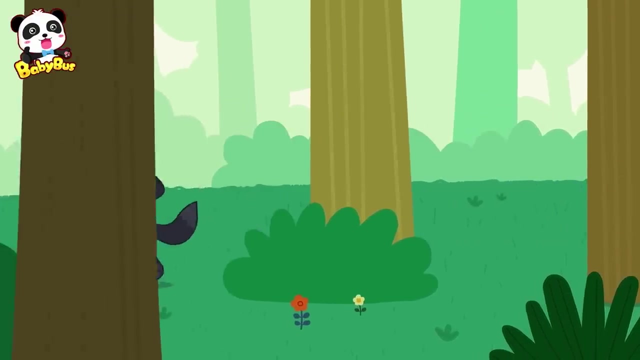 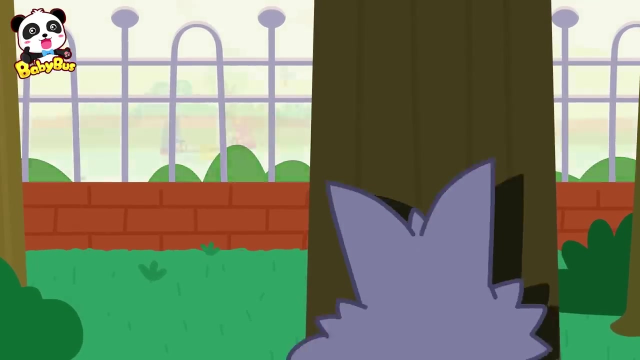 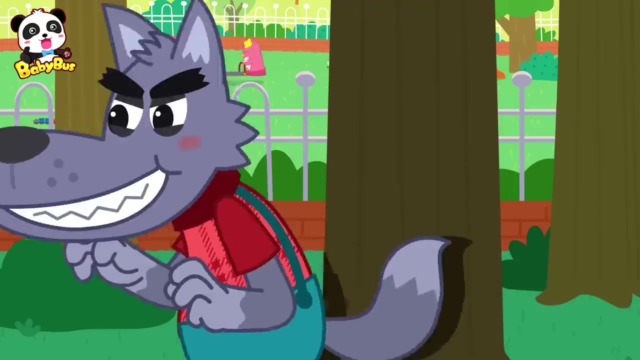 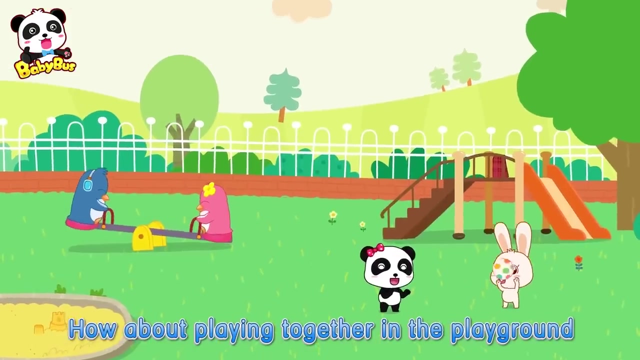 Do not panic And be prepared. Keep in mind The help will be here. Take cover, Earthquake, Earthquake, Earthquake. Don't panic. Take cover, Do not panic. If you're trapped, Stay calm, Don't be afraid, Stay calm, Stay calm, Stay calm, Stay cool. 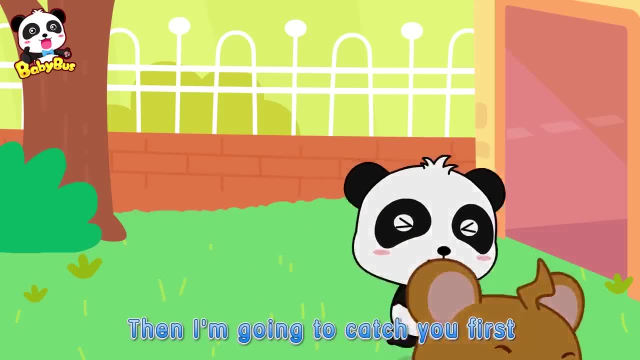 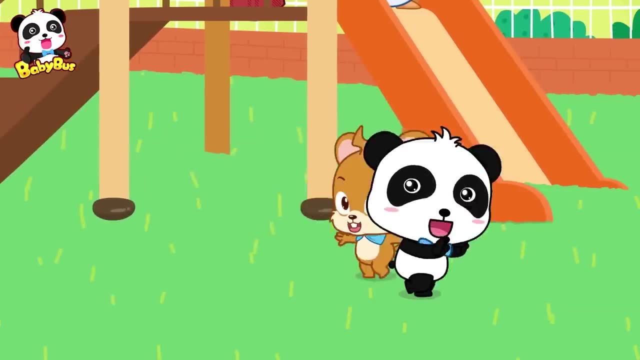 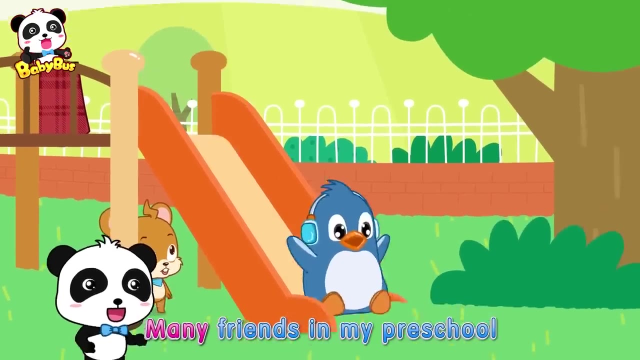 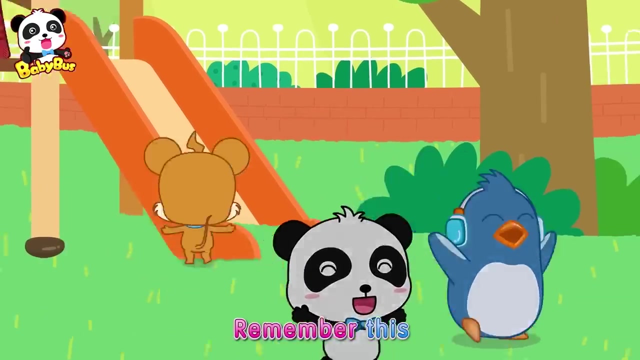 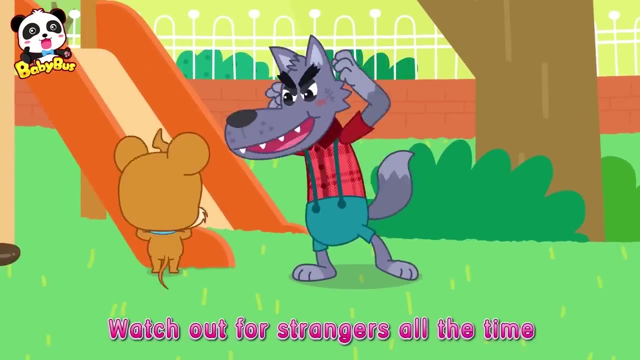 Stay calm, Stay calm, Stay calm, Stay cool, Stay cool, Then I'm going to catch you first. Many friends in my preschool. It's so fun to play with them. Remember this: please be safe. Watch out for strangers all the time. Who are you? 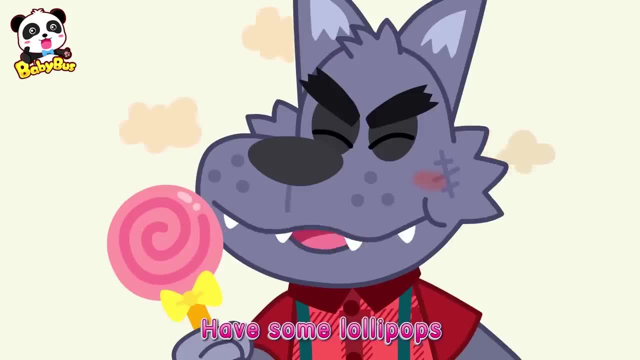 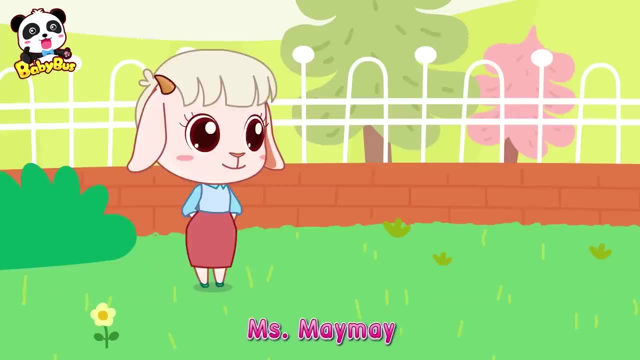 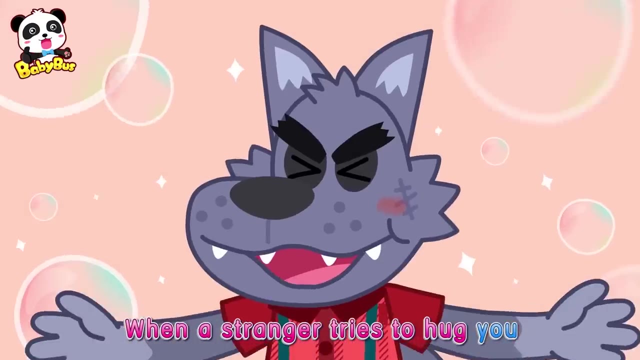 Little kid, come with me Have some lollipops. No, Our teacher told us not to take anything from strangers. Miss Mimi, there's a strange man here. When a stranger tries to hug you, Don't be afraid and shout out. no. 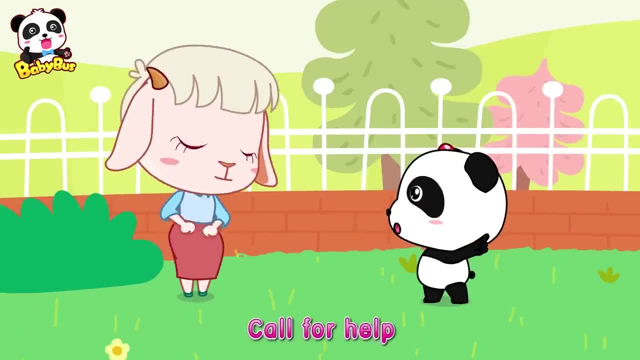 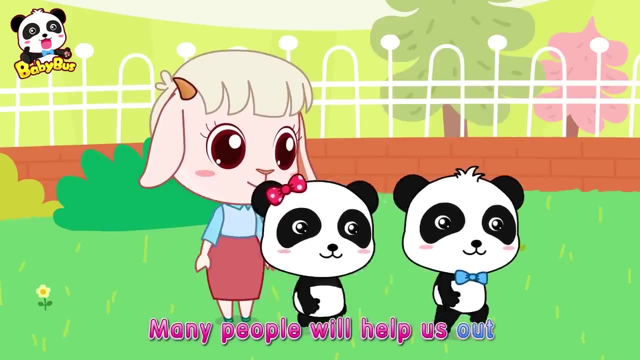 When you're in danger, call for help. Try to take care of yourself. Many people will help us out. The teacher and the security guard Ask for help at any time. Remember to protect yourself, please. The teacher and the security guard. 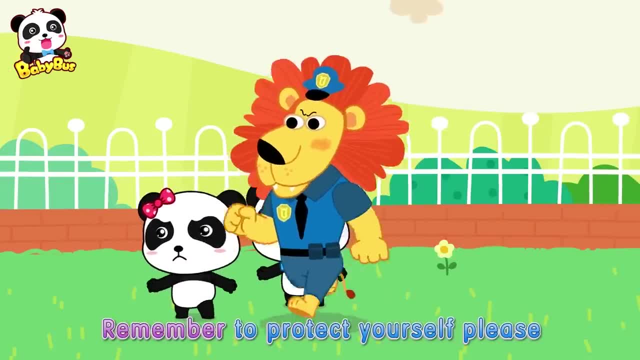 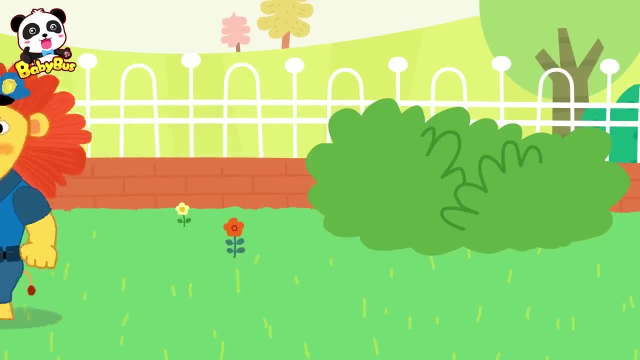 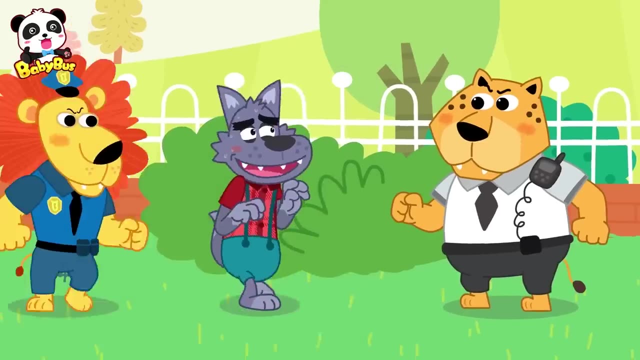 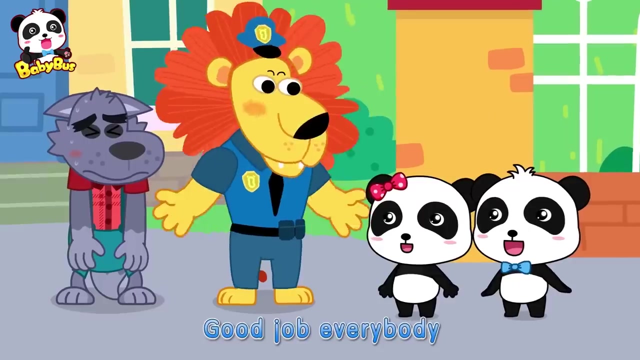 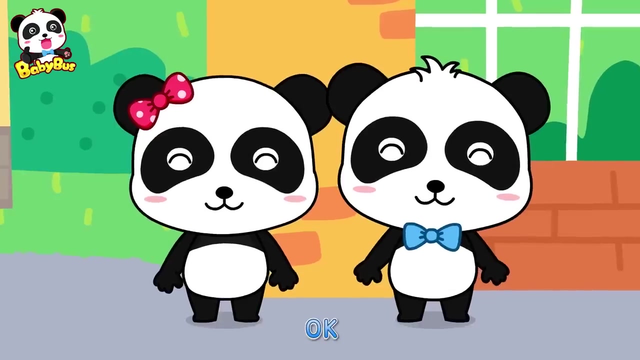 Ask for help at any time. Remember to protect yourself. please The teacher and the security guard. Ask for help at any time. Good job everybody. When you see a stranger around here, Tell your teacher immediately. When you see a stranger around here. 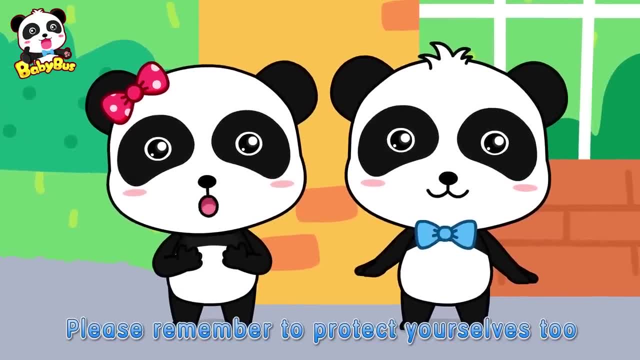 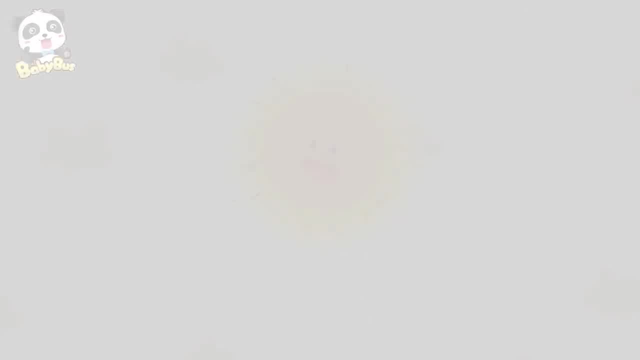 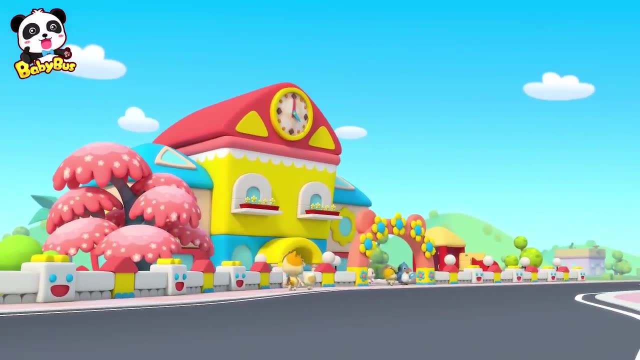 Tell your teacher immediately: Okay, we'll protect ourselves. Kids, please remember to protect yourselves too. Kids, please remember to protect yourselves too. Kids, please remember to protect yourselves too. Mom, Timmy, Timmy, let's go home. 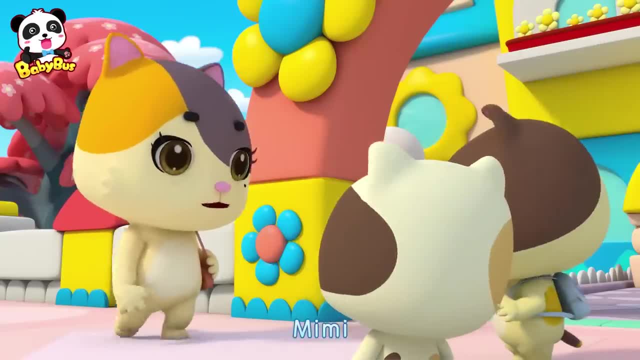 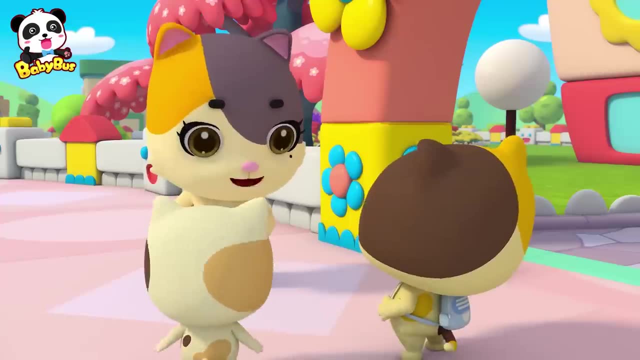 Timmy, let's go home, Mimi, we'll go to the supermarket first. Wow, I love the supermarket, Mimi. the supermarket is across the street. Mimi, the supermarket is across the street. Do you know how to cross the street safely? 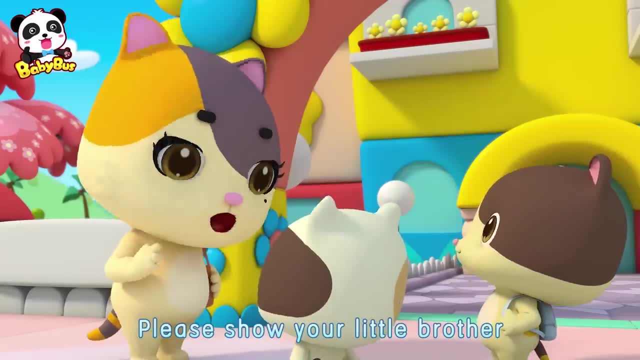 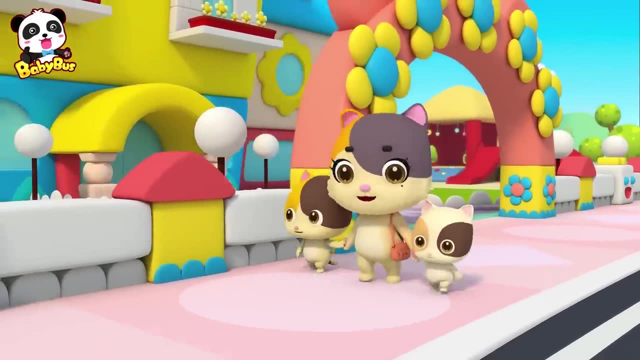 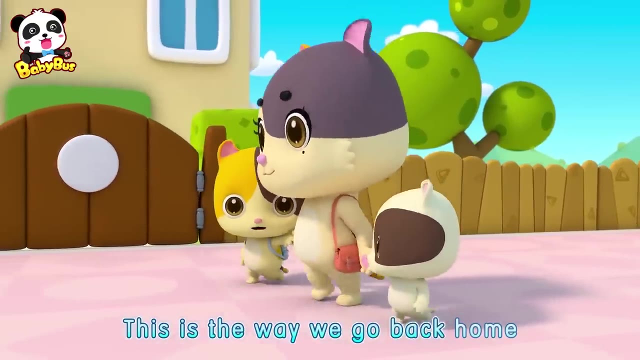 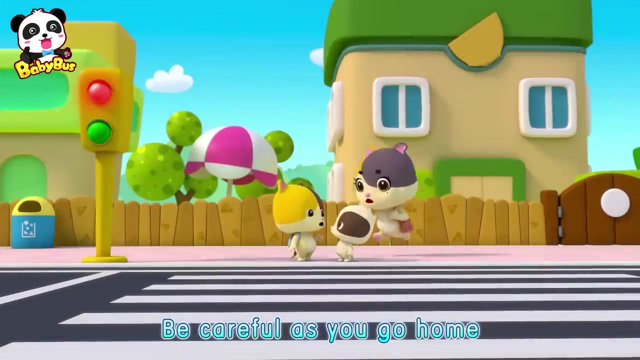 Sure Good, Please show your little brother how to do it. Let's go, Let's go. This is the way we go back home. Go back home, go back home. Be careful as you go home. This is the way we hold our hands. 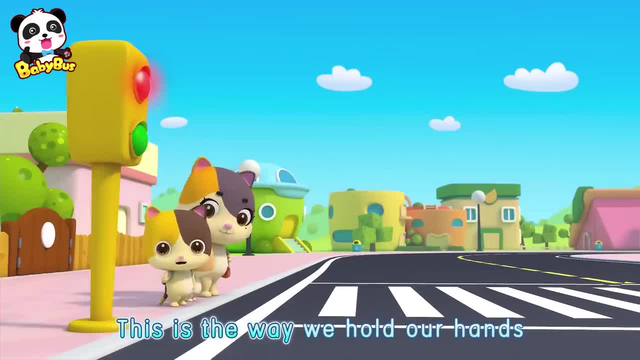 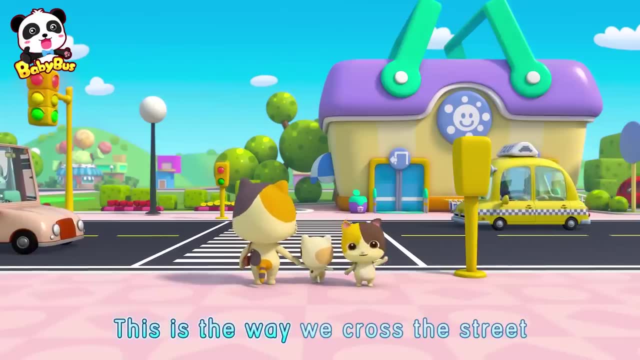 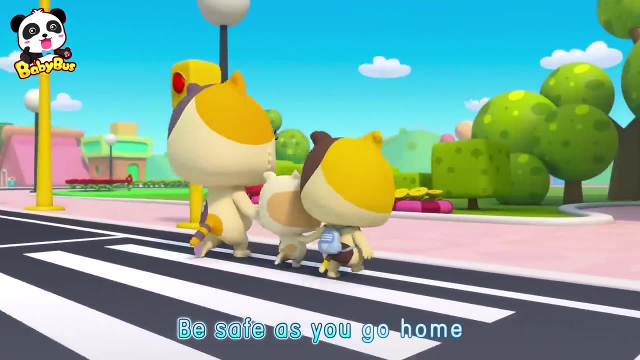 Hold our hands. hold our hands. This is the way we hold our hands. Be careful as you go home. This is the way we cross the street. Look to the left, look to the right. This is the way we cross the street. Be safe as you go home. 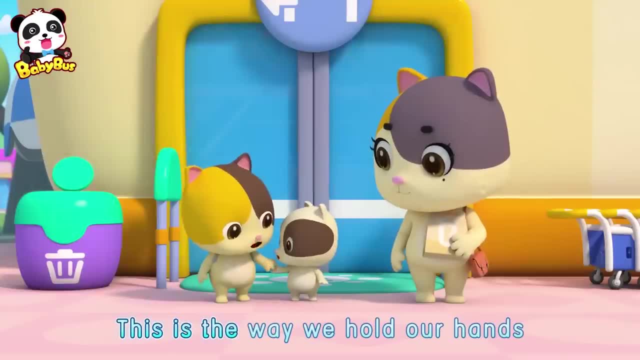 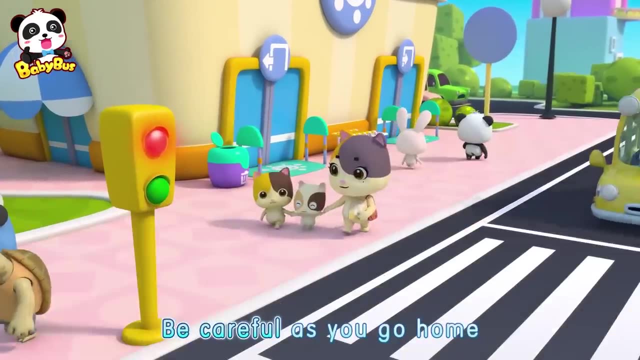 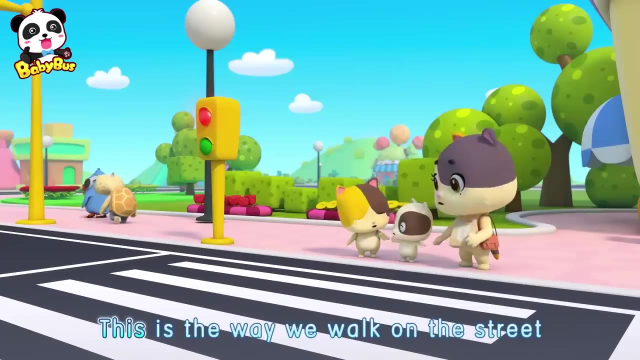 Yeah, here's the supermarket. This is the way we hold our hands. Hold our hands, hold our hands. This is the way we hold our hands. Be careful as you go home. This is the way we cross the street. Never run, never run. This is the way we walk on the street. 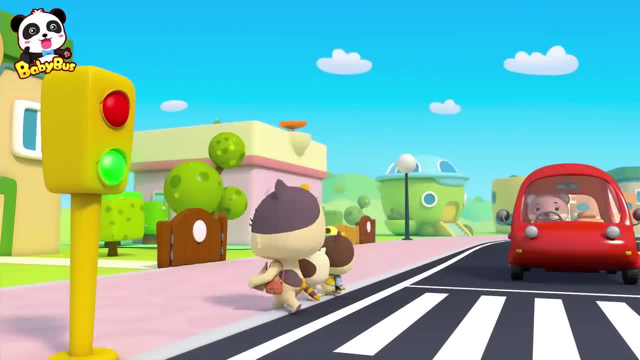 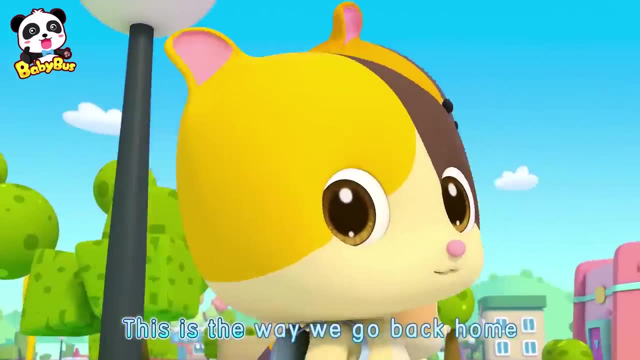 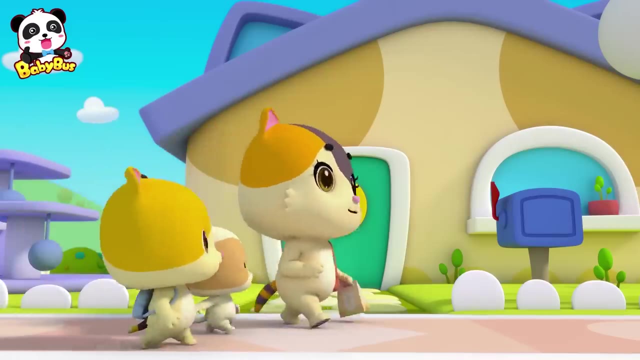 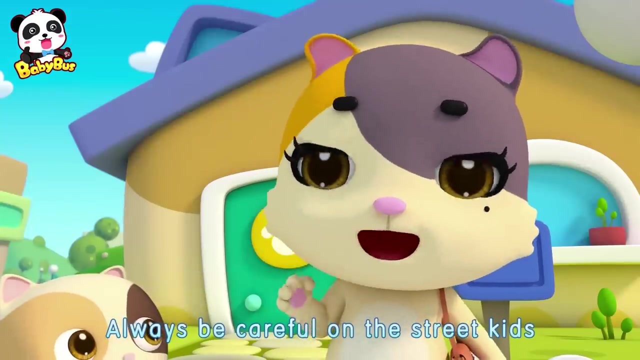 Be safe as you go home. This is the way we go back home. Hold our hands, hold our hands. This is the way we go back home. We are home safe and sound. We're home. Yeah, Always be careful on the street, kids, So that you can get home safely. 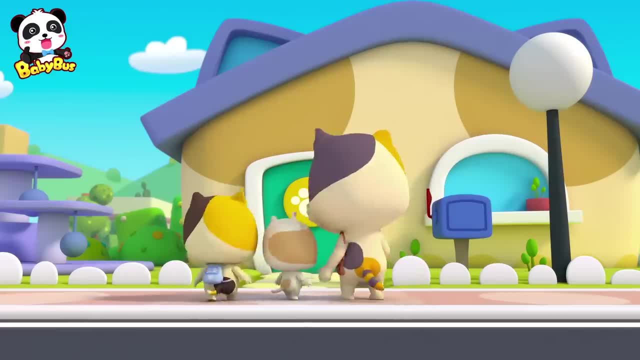 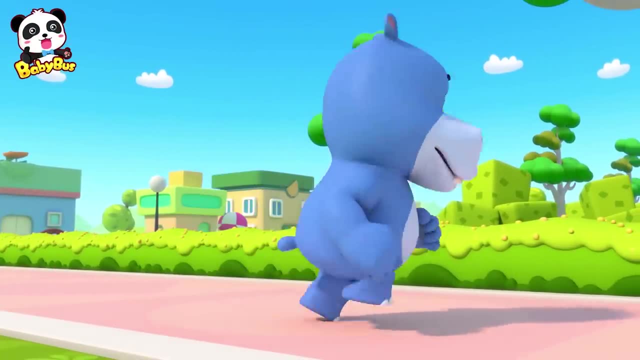 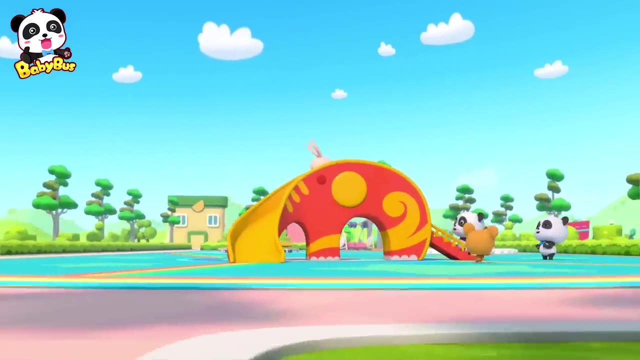 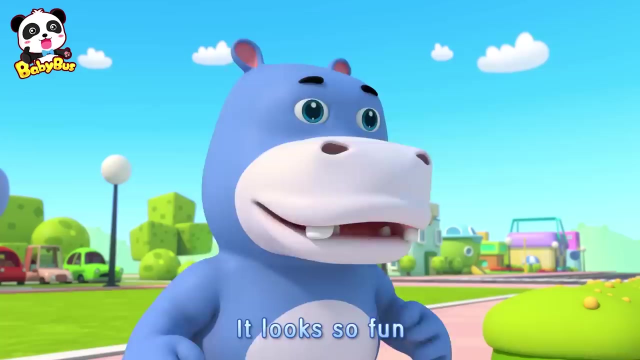 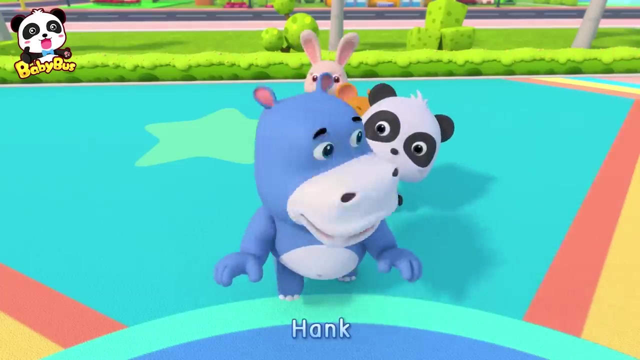 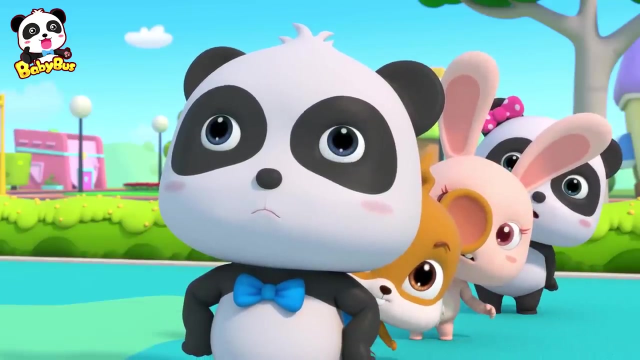 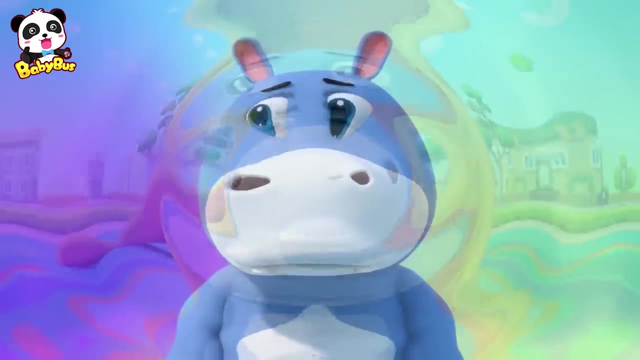 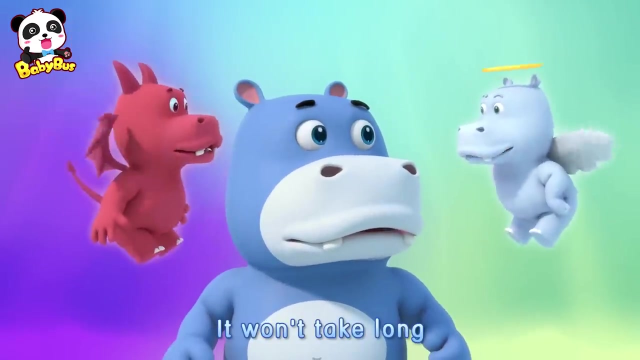 Yeah, Always be careful on the street. Hang, you should line up first. Why do I have to? I want to ride the slide now. You don't have to. You can ride the slide right now. It won't take long. If you line up, everyone can have fun together. 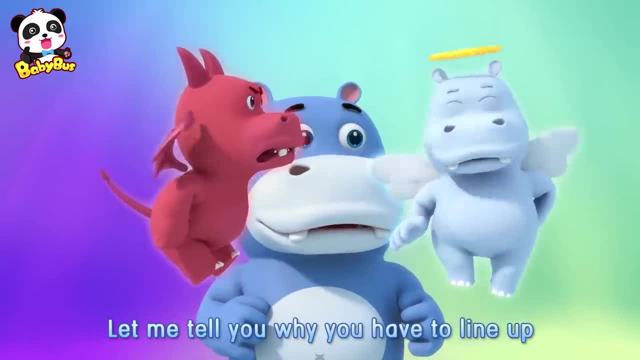 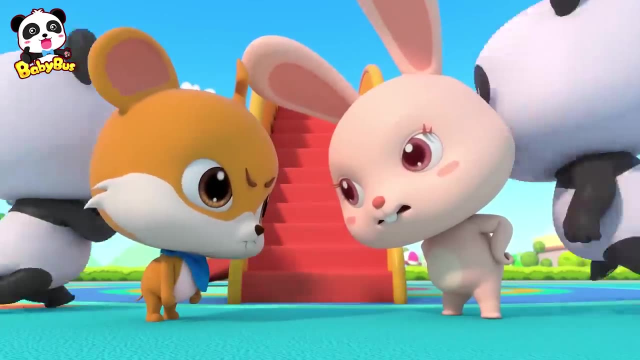 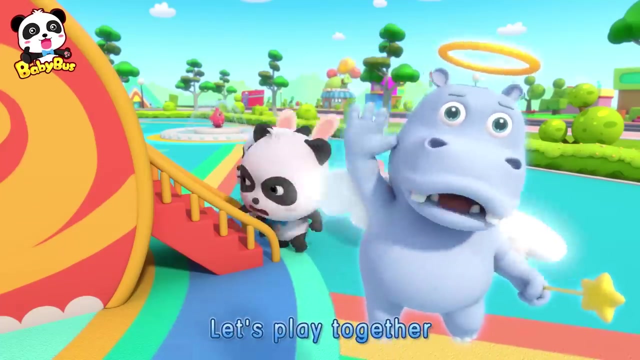 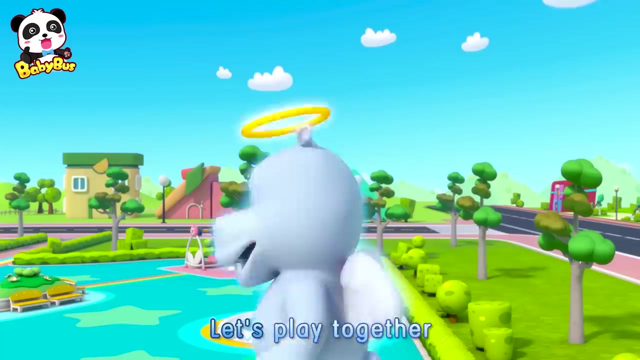 Don't line up. Let me tell you why you should line up, Why You have to line up. Let's play together. Do not push your friends. Line up, oh, line up, Have fun now. Let's play together. Let's play together. Stand in line and wait your turn. 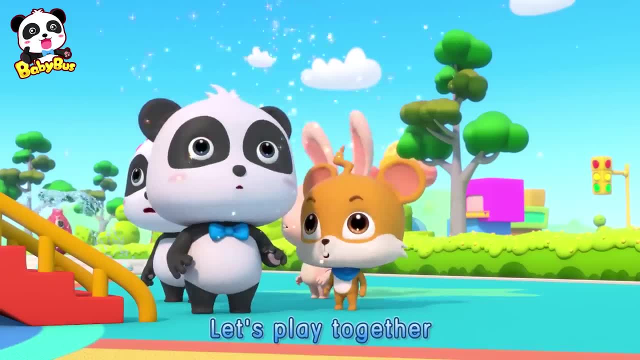 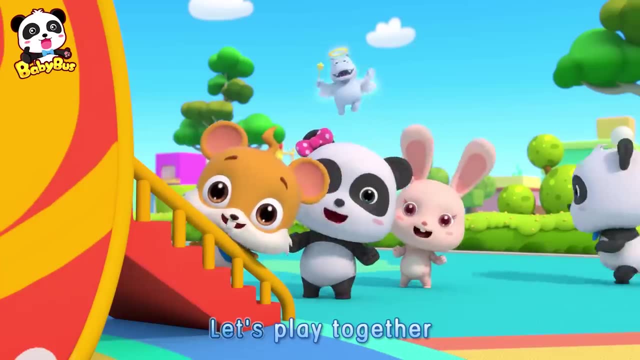 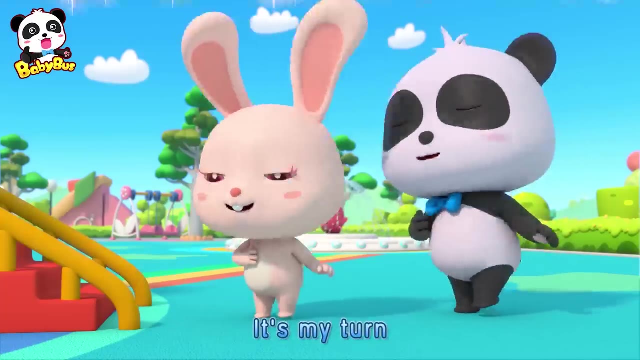 Stand in line and wait your turn. Let's play together. Stand in line and wait your turn. One and then another. Let's have fun. Let's play together. Please wait, don't be angry. Next one and next one. It's my turn. Let's play together. Do not push your friends. 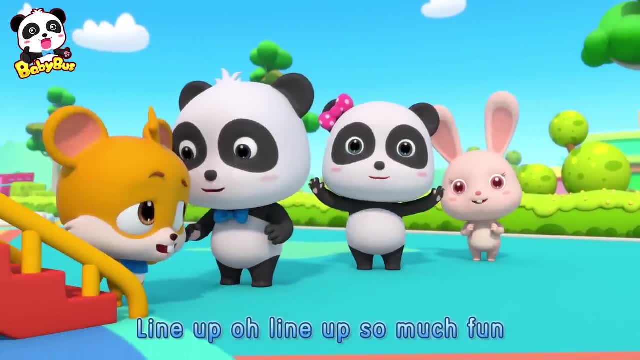 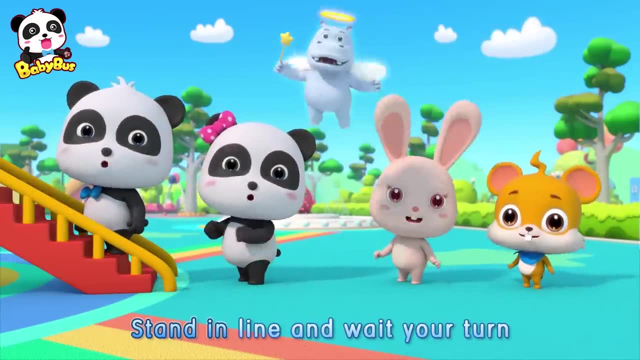 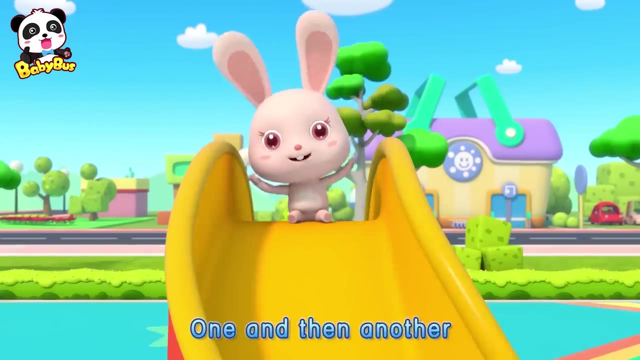 Line up, oh line up. So much fun. Let's play together. Let's play together. Stand in line and wait your turn. Stand in line and wait your turn. Let's play together. Stand in line and wait your turn. One and then another. Let's have fun. Let's play together. 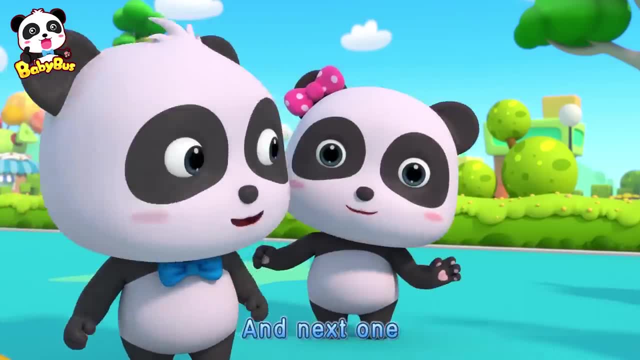 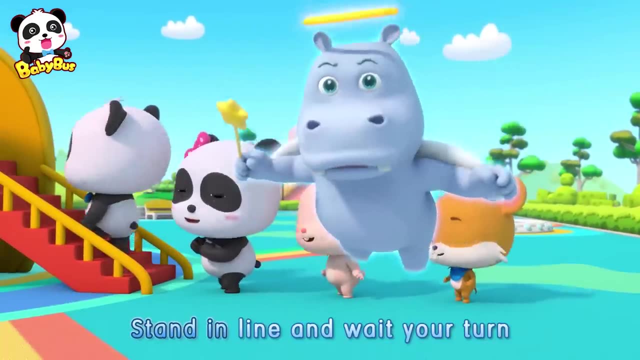 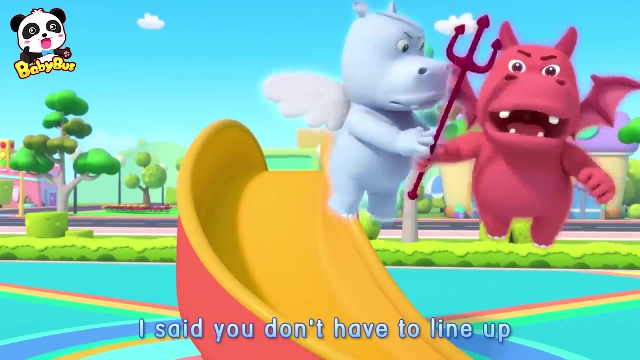 Please wait, don't be angry. Next one and next one. It's my turn. Let's play together. Let's play together. Stand in line and wait your turn. You can have so much fun. You can have so much fun. I said you don't have to line up. 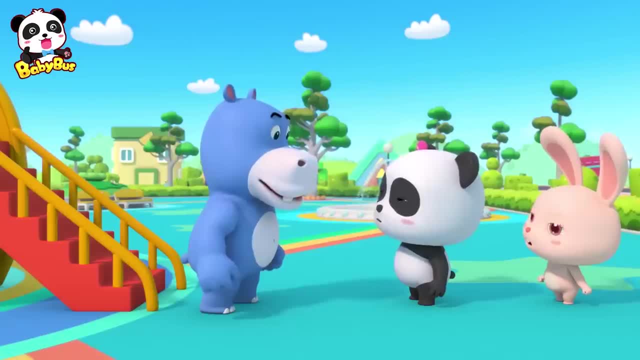 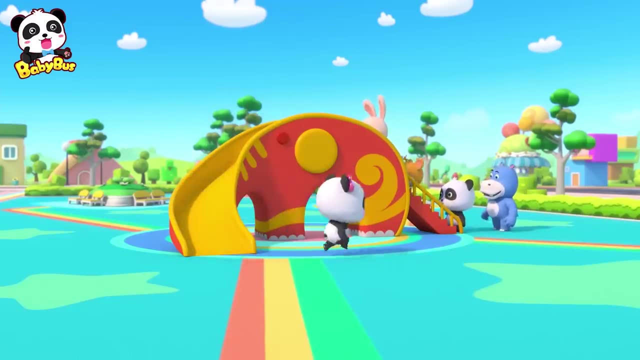 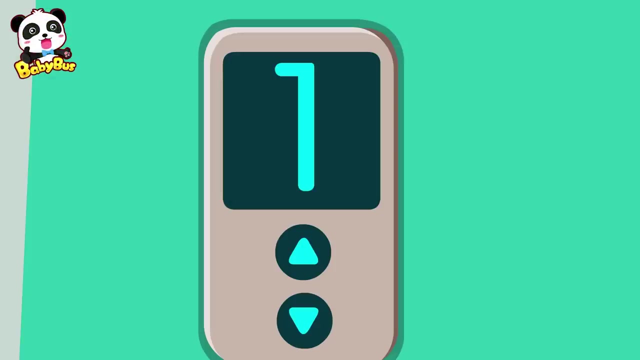 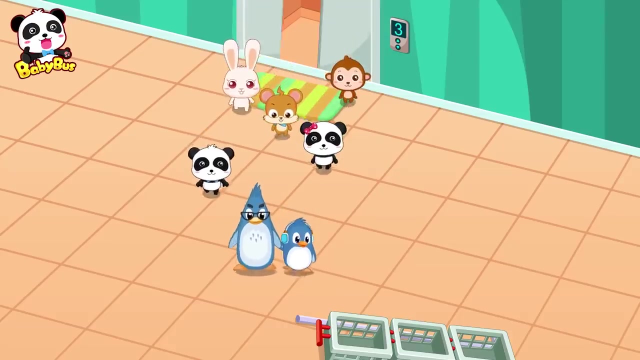 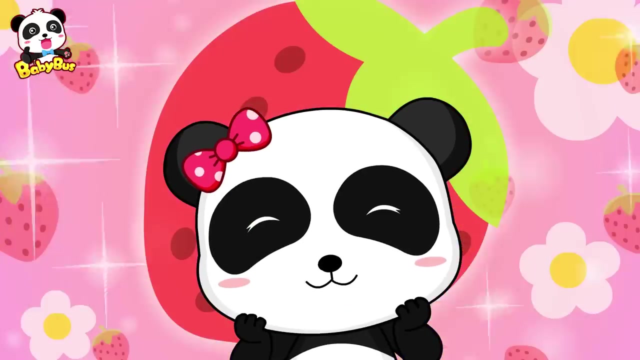 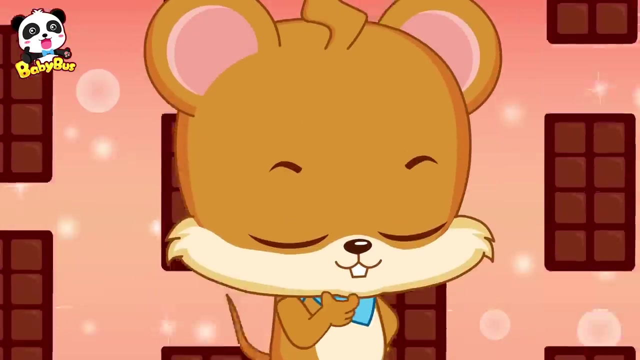 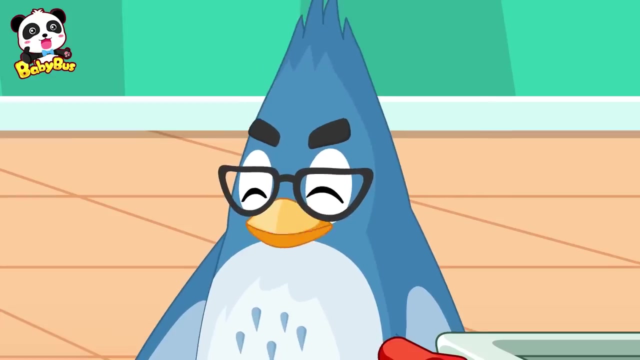 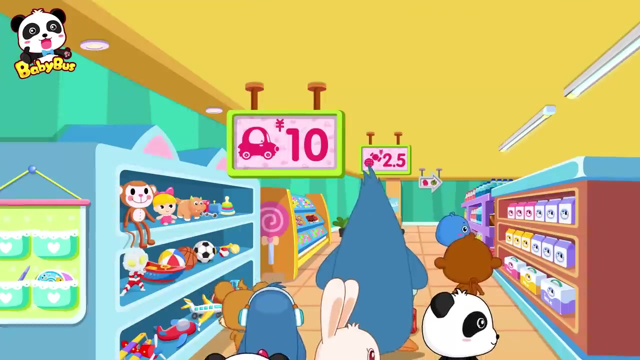 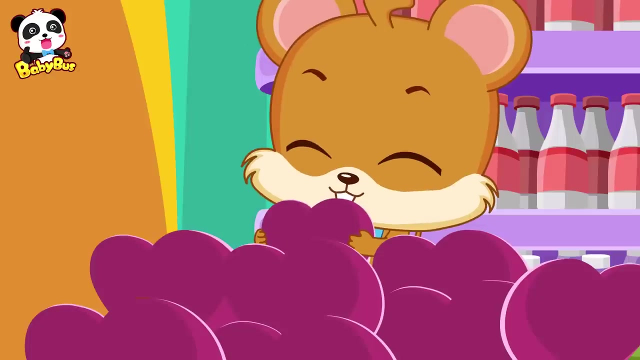 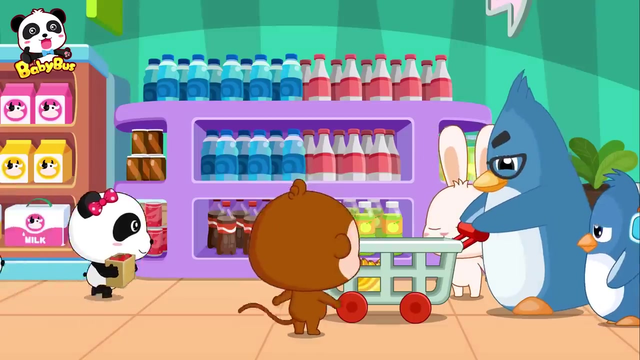 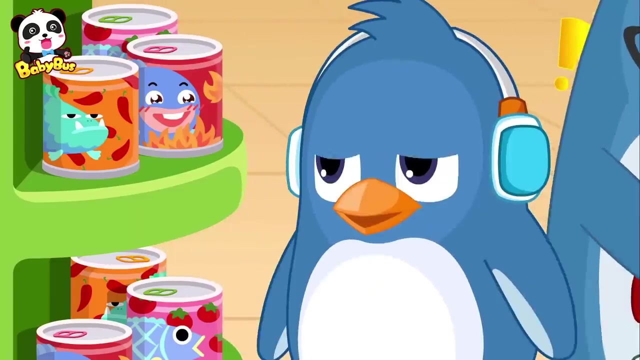 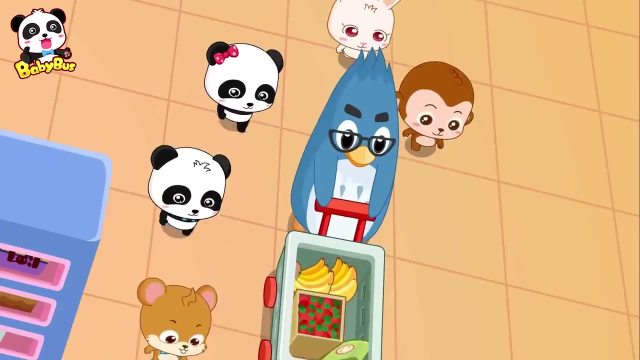 Alright, I will line up. Alright, I will line up. Yeah, What to do if you get lost Kids. what do you want for the picnic tomorrow? What do you want for the picnic tomorrow? Okay, here comes the shopping cart. Hmm, tomato sauce or soy sauce? 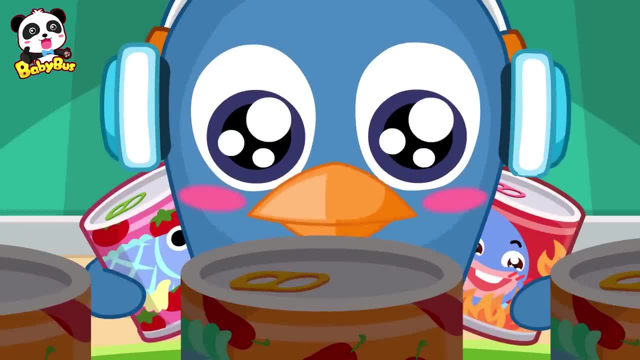 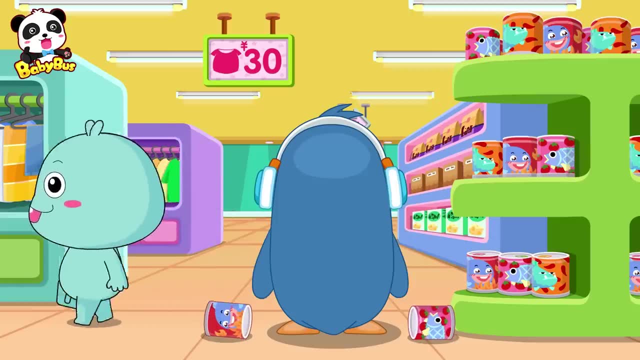 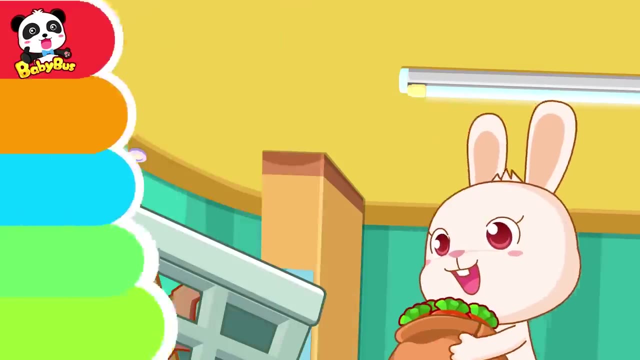 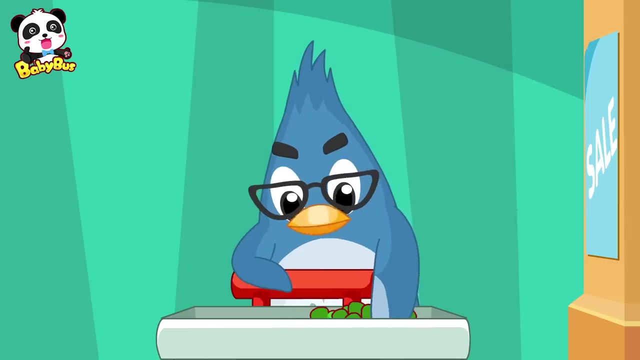 Or should I say tomato sauce? Or should I choose a spicy one, Dad? which one should I choose? Huh, Dad, Kiki, Mew Mew, Where have you gone? Let me see what you all have bought. Rudolph, did you get your favorite canned fish? 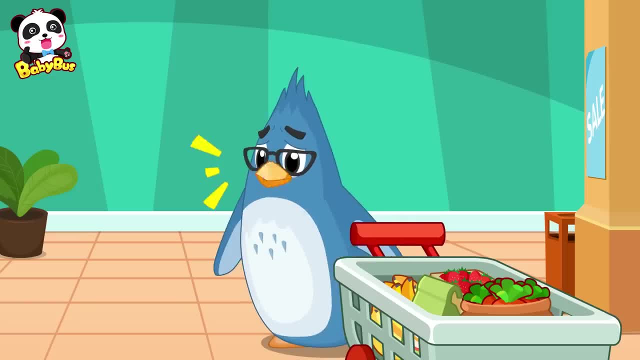 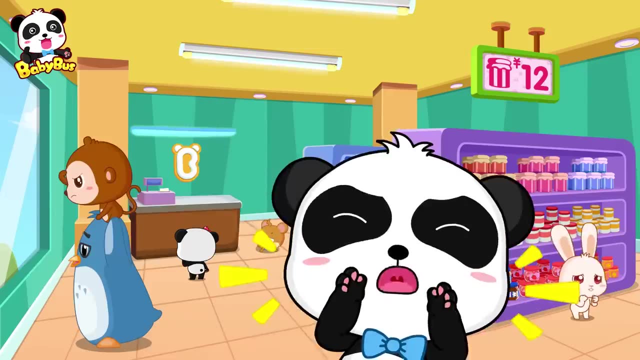 Huh, Huh, Rudolph Rudolph, where are you? Rudolph's missing Rudolph, Rudolph Rudolph, Where are you? Rudolph, where are you? You guys stay with me, don't run away. 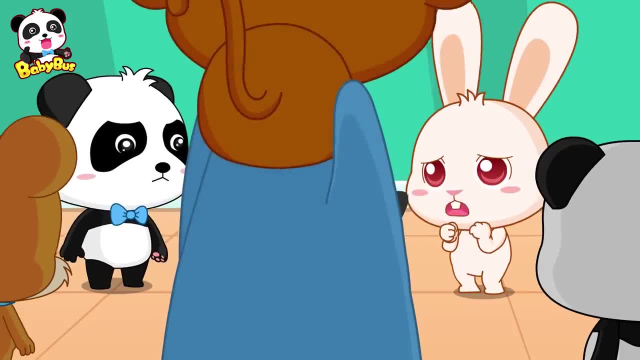 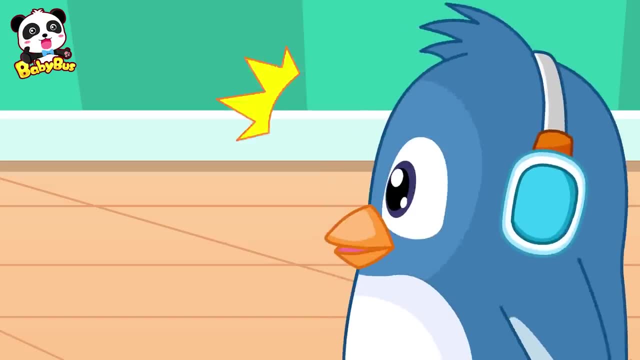 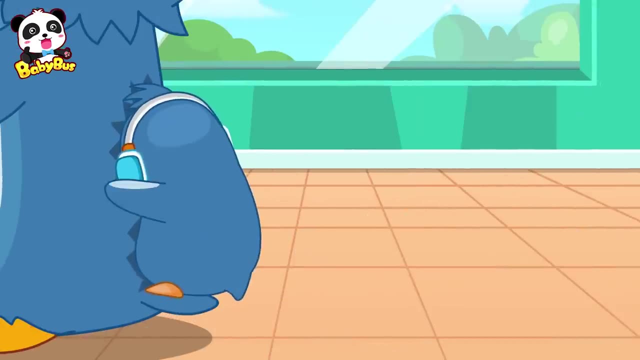 Otherwise someone else will get lost too. Oh, my goodness, Rudolph must be desperately looking for us. There's Dad. Dad, I thought I lost you. Oh, I'm sorry, I made a mistake. Dad, where are you? Remember your parents' phone numbers? 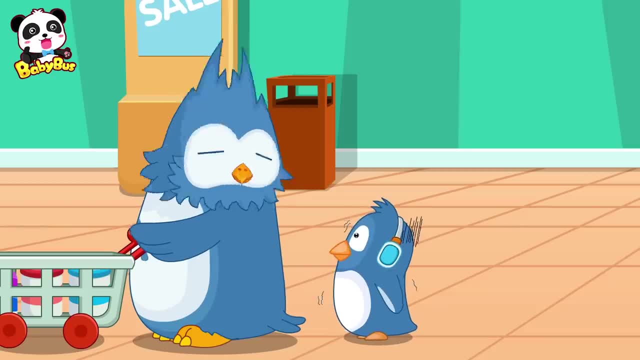 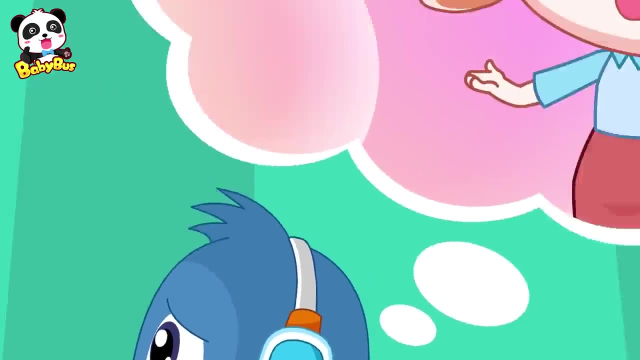 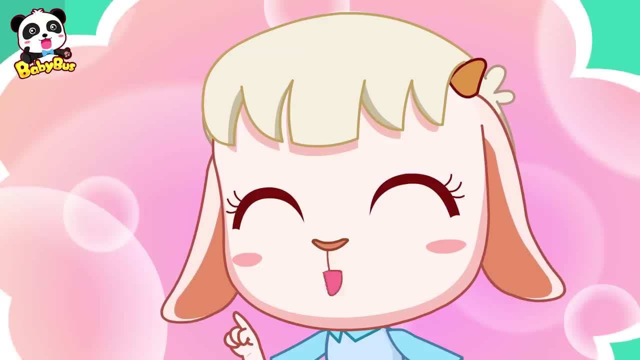 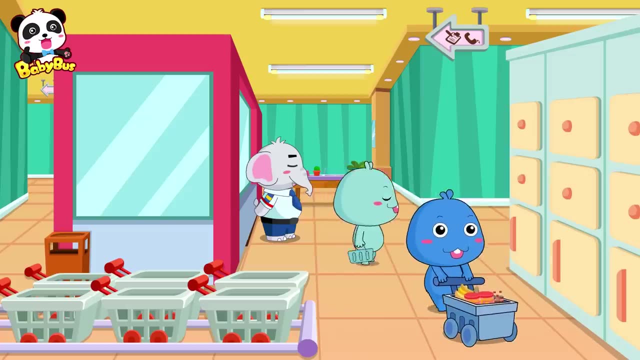 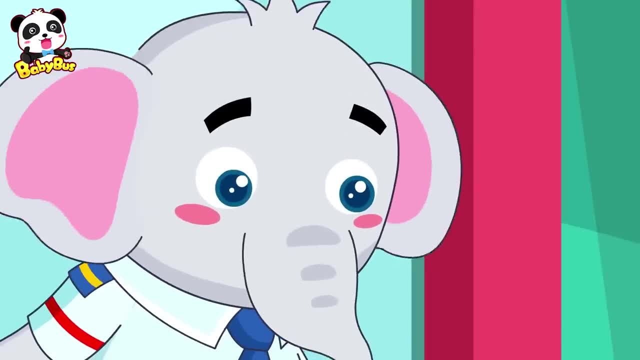 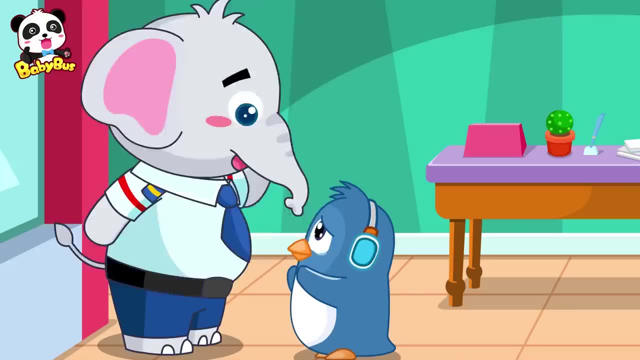 Huh, Huh Huh. Hello son, Are you alone? Have you gotten separated from your parents? I lost my dad. I can't find him. What's your name? Rudolph Rudolph. do you know your dad's phone number? 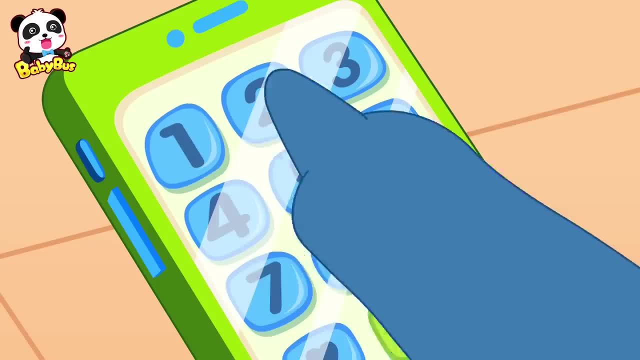 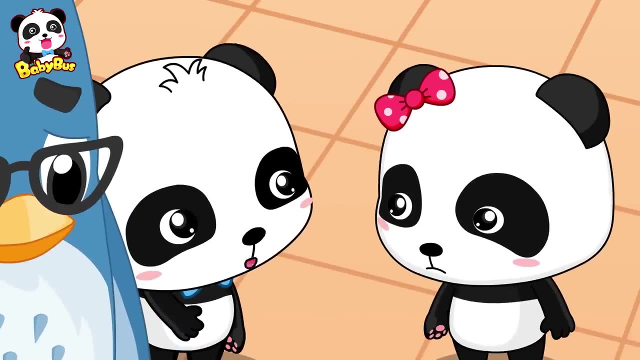 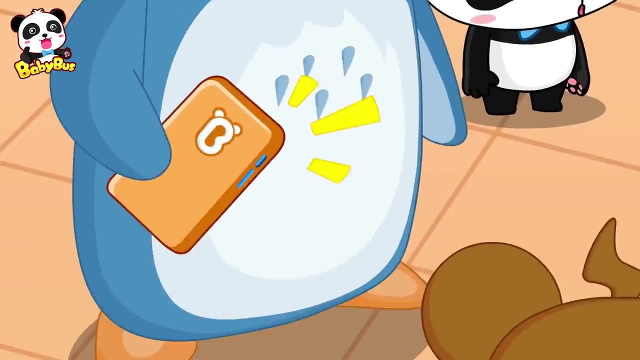 Yes, I do. 1-8-1-2-0-8-2-1-8-5-8, Miu, Miu, let's ask Du Du to find Rudolph. Good idea, Hello Dad, it's me Rudolph. 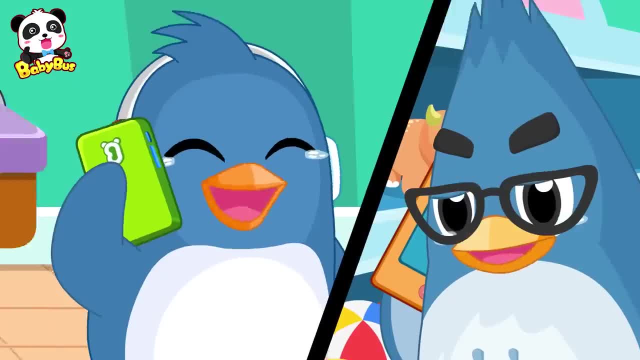 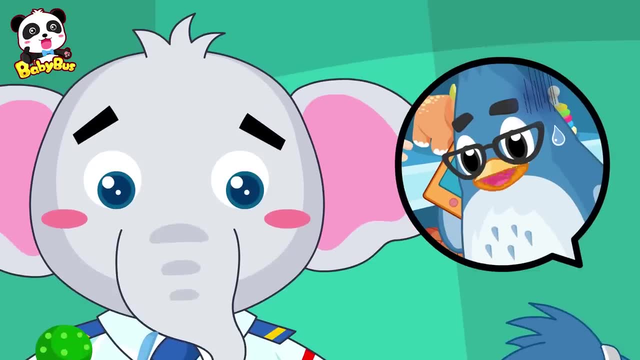 Rudolph, It's Rudolph, Yay, Where are you now? I'm next to a table- A table, What else do you see? And a security guard is here. Rudolph, give the phone to him. Let me talk to the security guard. 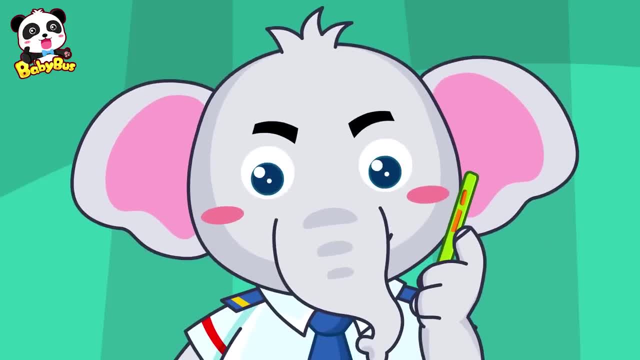 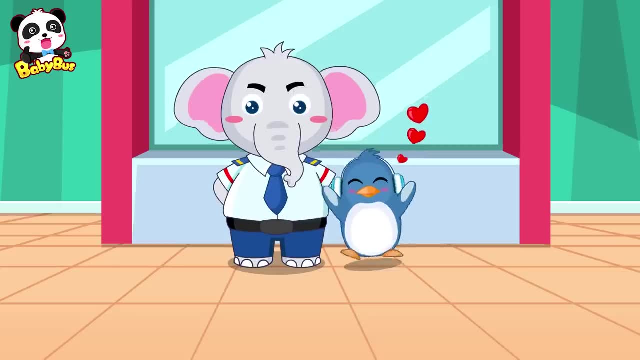 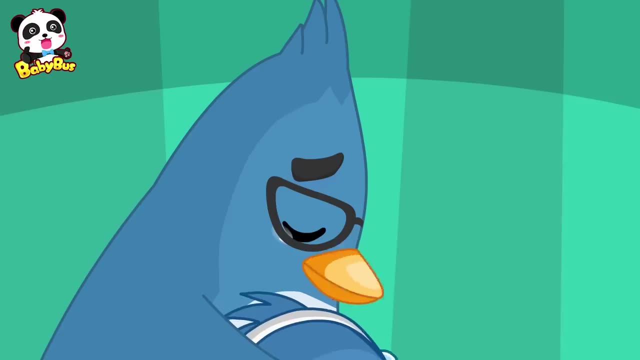 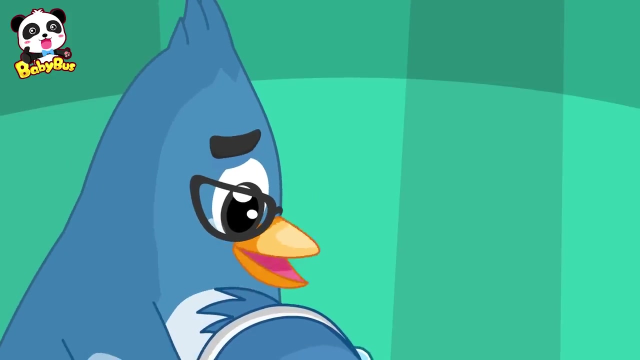 Okay, Uh, hello, Your son and I are at the supermarket entrance. Hey, there's Rudolph. Ah, Dad, Dad, Dad, Rudolph, it's okay now Stay close to me next time. Thank you so much, Rudolph. thank the security guard. 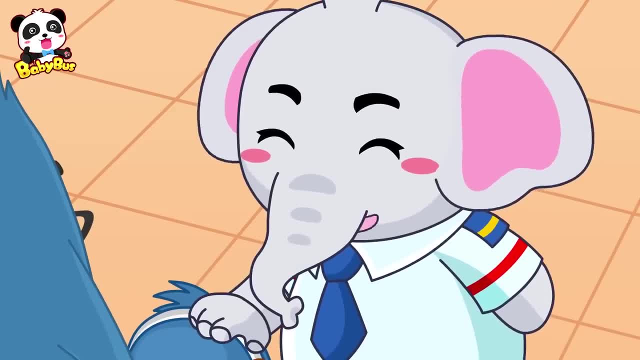 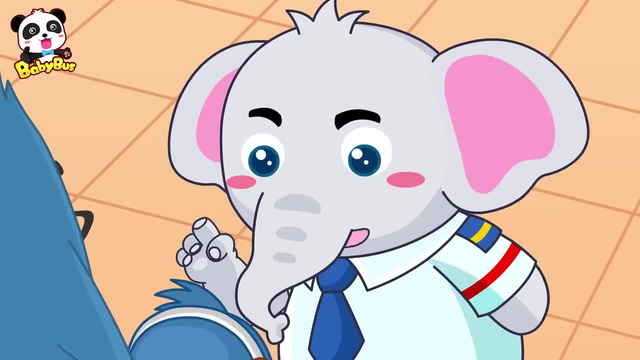 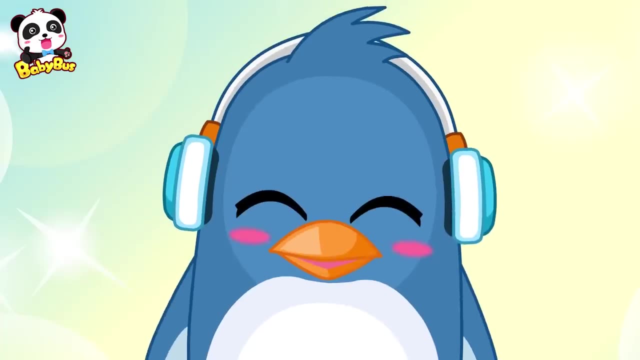 Thank you, sir. You're welcome. Rudolph, you did well. You stayed calm, came to me for help And remembered your dad's phone number. Rudolph, it's good to see you. We were worried about you. We were so worried about you. Hey kids, if you get separated from your mom and dad, 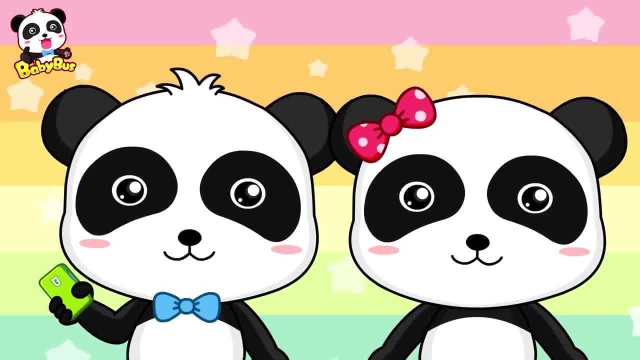 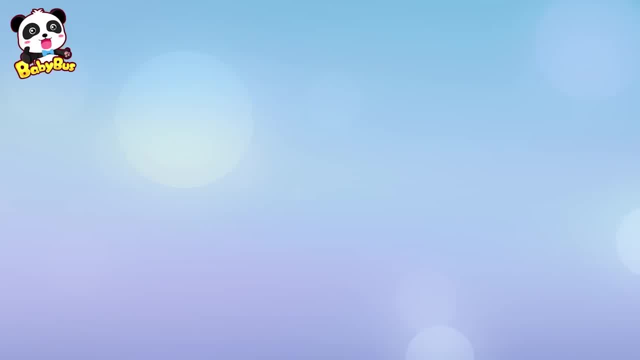 Go to find a security guard And memorize your mom and dad's phone numbers. Yeah, Rudolph, you do it. Goodbye. What, Rudolph, about the house? I can't come back. I have no idea. I feel bad. Rudolph, you're going to hell.